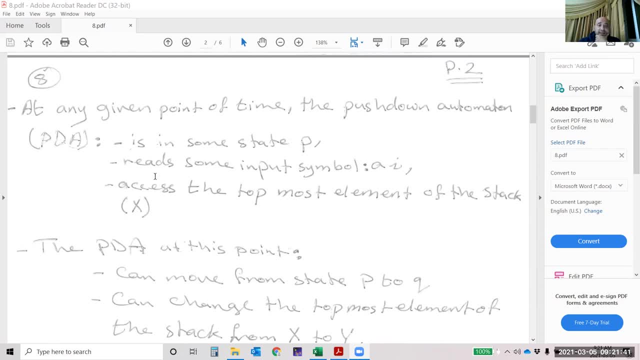 At any given point of the time. the push-down automaton PDA is in some state at that time, should be in some state. P read some input, simple AI access, the topmost element of the stack X: either push or pop. 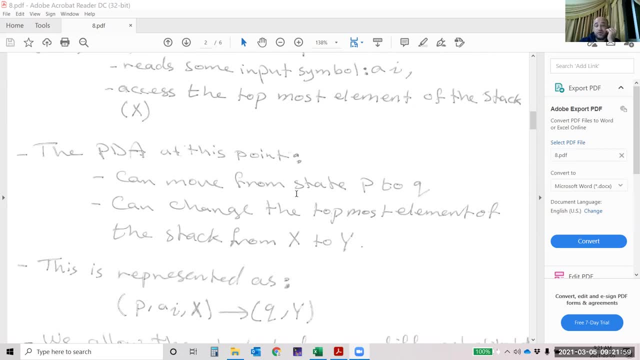 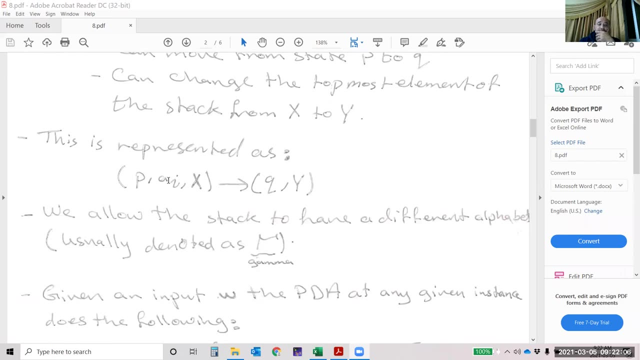 The PDA at this point can move from state P to Q, can change the topmost element of the stack from X to Y, for example. This will be represented that we put the P- the name of the state, what is the symbol read and what we will push on the stack and what will be replaced, which state I will be and what is the symbol that I push it in the stack. 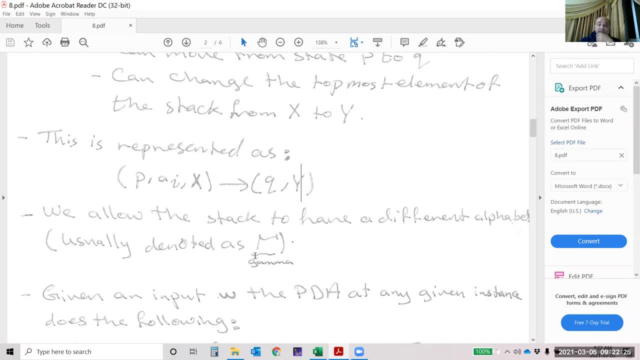 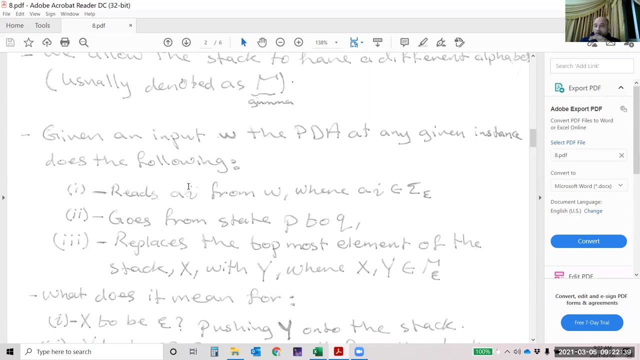 We allow the stack to have a different alphabet usually denoted, as yesterday I said, draw it's gamma, it's gamma capital in Latin. So this is gamma capital, gamma, Given an input W. the PDA, at any given instance, does the following: We talked all about this yesterday and I'm repeating this in the class note: 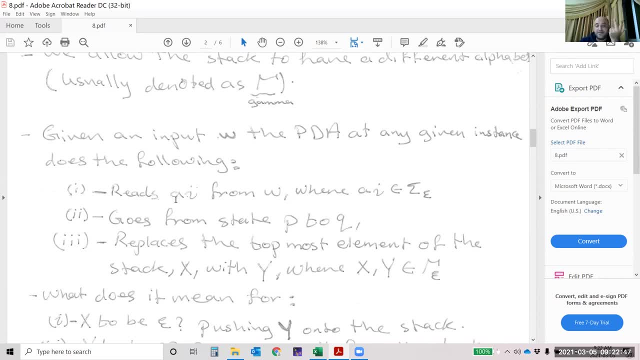 We will read AI from W, where AI belongs to, sigma epsilon goes from state P to Q. replaces the topmost element of the stack, X with Y, where X and Y both are elements of the stack alphabet. Gamma epsilon is the stack. 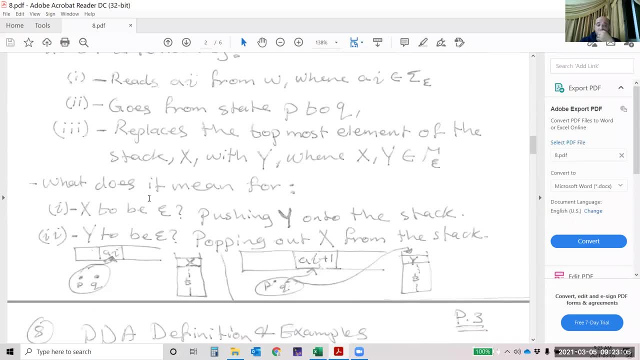 What does this mean? What does this mean for X to be an epsilon or Y to be an epsilon? If X is an epsilon, then we're pushing Y on the stack immediately. We don't need to pop anything. If Y to be an epsilon, popping out X from the stack. 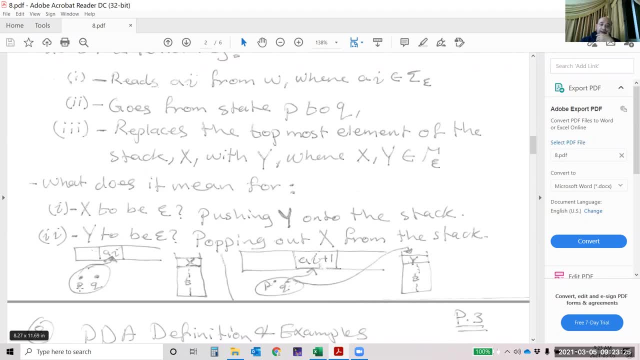 We have to take out X from the stack. So, for example, if I'm at state P and I read AI and I have X, then I'll I'll read. it asks me, for example, to either leave X and become below Y or pop it out. 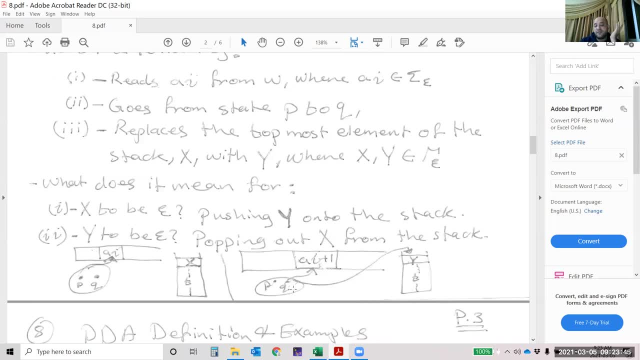 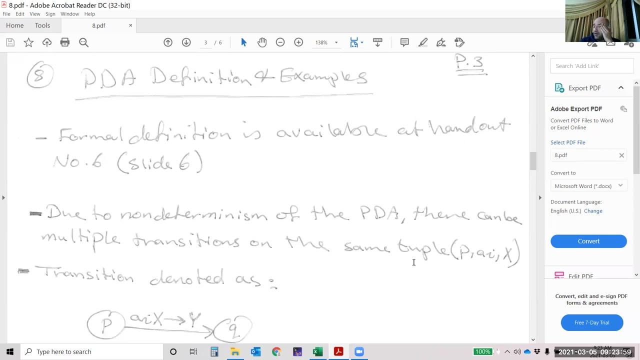 Doesn't matter, depends on the state. So I move from state P to state Q, The pointer now at symbol AI plus one. the next symbol, and Y become the top of the stack or the topmost element. Example: formal definition of the PDA. we have it yesterday in handout six. 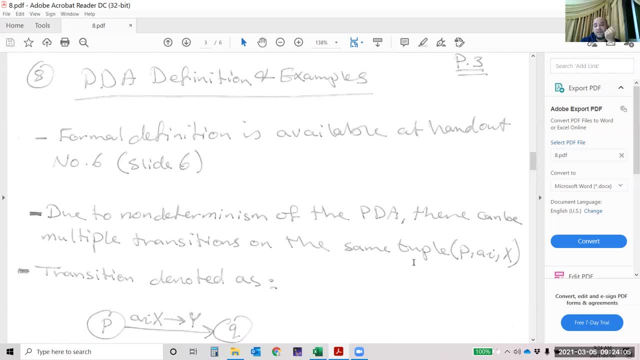 Slide six: due to the nondeterminism characteristic of the push down automaton, there can be multiple transition on the same tuple- P, AI and X- And we'll see some example. we'll make some branches, because I have two scenarios: case one, case two. 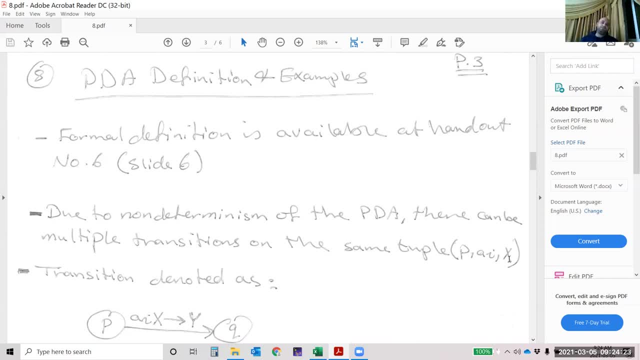 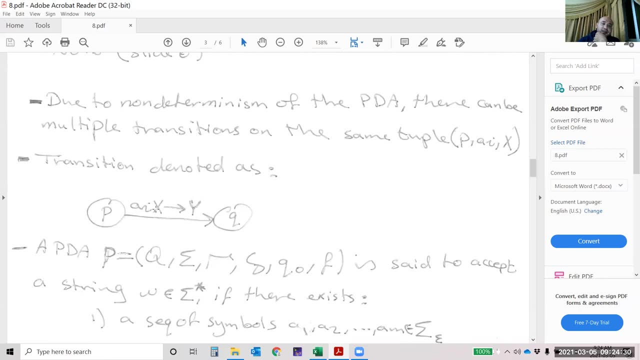 So we can go in both direction. So the transition denoted: I'm at state P, I read AI and there is X. So I'm at state P, I read AI and there is X. So the transition denoted: I'm at state P, I read AI and there is X. 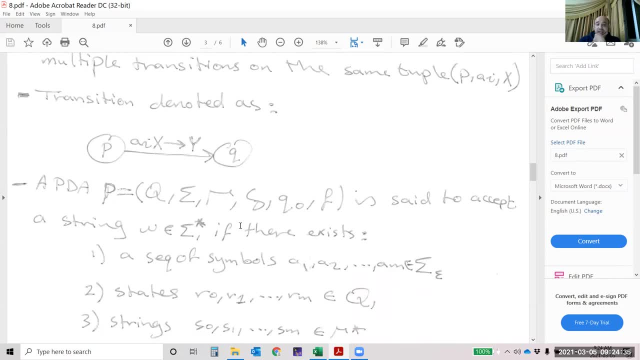 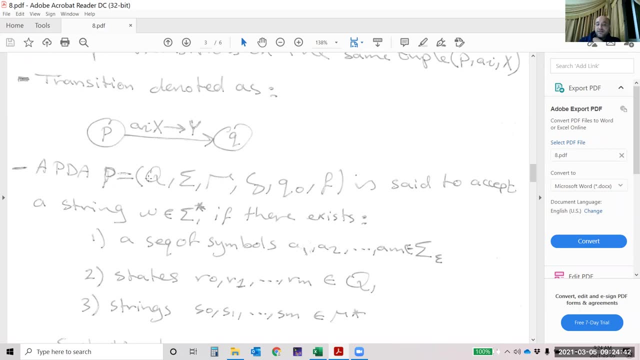 So the transition denoted. I'm at state P, I read AI and there is X And replace it with Y and I move to Q. As we saw yesterday that the PDA consists of a tuple: Q, which is the set of states, sigma, which is the alphabet, gamma, which is the stack alphabet, delta, which is the transition function, and the Q node, starting state, and F is the accepting state. 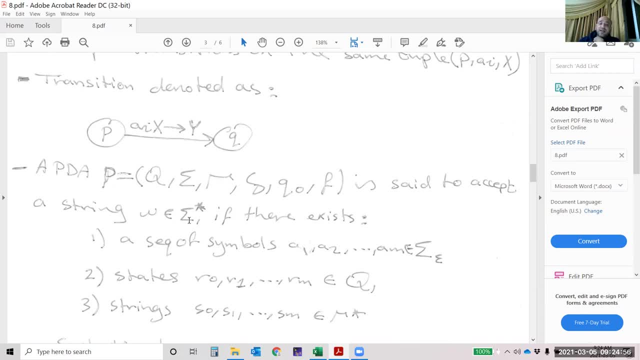 It's said to accept a string W that belongs to sigma star. if there is, exist A sequence of symbol A1 to AM that belongs to sigma star. A sequence of symbol A1 to AM that belongs to sigma star. A sequence of symbol A1 to AM that belongs to sigma star. 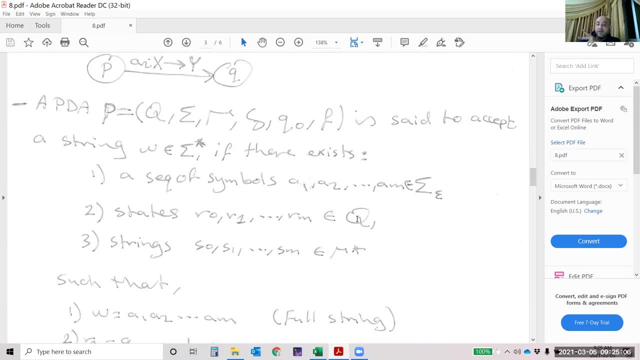 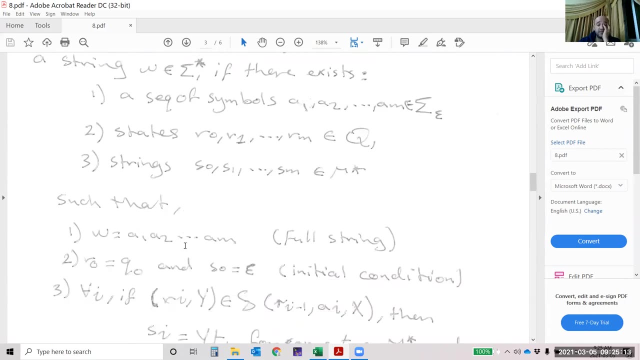 State R0, R1 to RM that belongs to Q, and the string S0, S1 to SM that belongs to the gamma star, which is the stack alphabet, Such that W- it's a full string- consists of different symbol from A1 to AM. 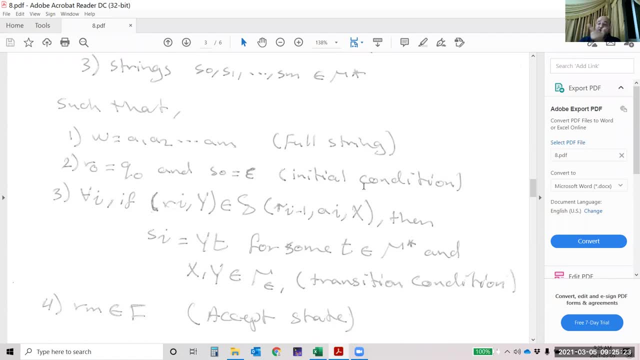 R0 is a Q node and S0 is epsilon initial condition for the stack For every I. if R, I, Y belong to delta, which is the transition function Of R, I minus 1, A, I and X, then S I will become the Y T. 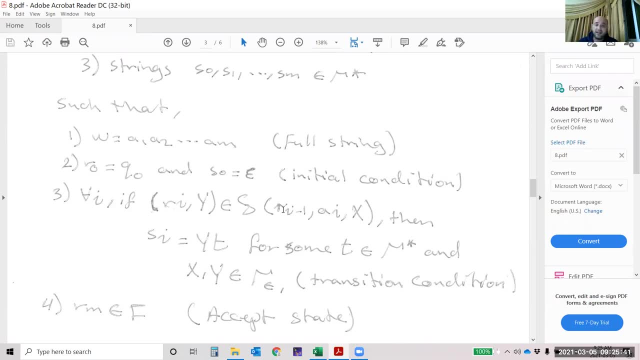 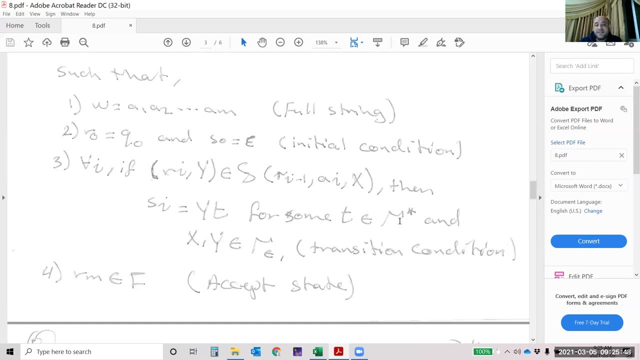 T. here we represent the remaining of the stack. T here in our drawing means the remaining stack contents. For some, T belongs to gamma star and XY belongs to gamma epsilon transition condition, RM. when I reach to RM, which belongs to F, which is the final state or accepted state, we are at accepted state. 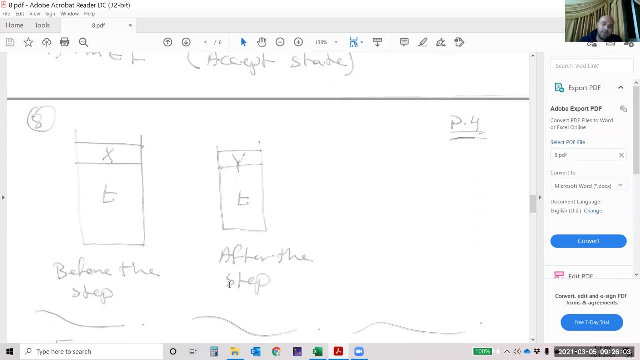 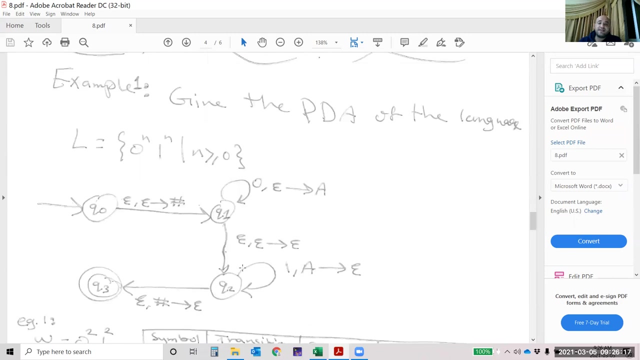 Otherwise reject Here in a vector form like X, T is the remaining of the stack before the step. After doing the step, Y becomes the top of the stack and T is the remaining stack contents after the step. So let's have an example same as our example yesterday. 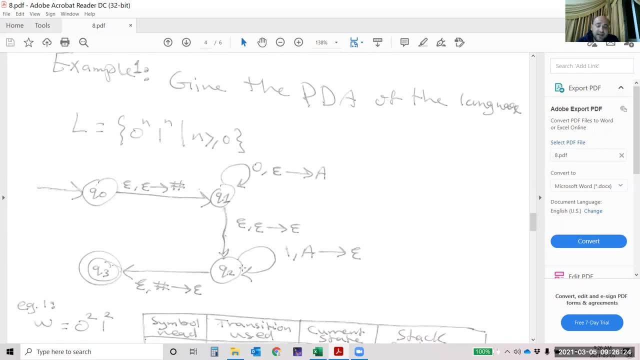 I will repeat it so to make sure that everybody is understanding it: Giving that the PDA push down automata of the language: L0 to the power N, 1 to the power N Where N is greater or equal to 0.. 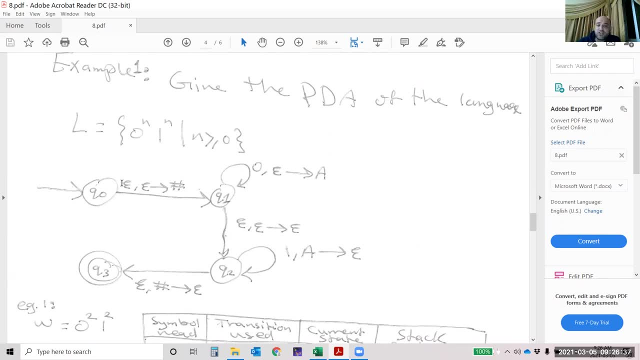 I'll start at start static QNOT With epsilon transition. I will push a hash in the stack. This: if you remember, in our handout we used the dollar sign. You can use any symbol for you. This symbol will let you know that I reached to the end of the stack. 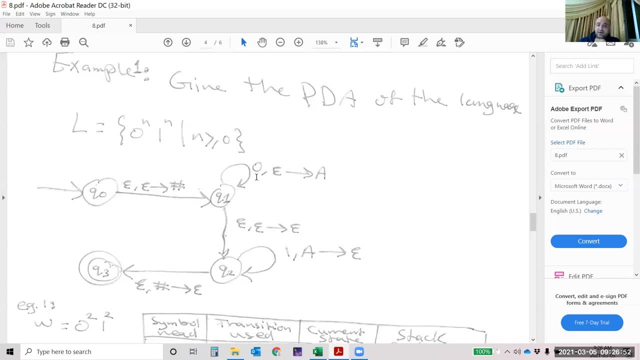 The stack now is empty. So if I receive a 0, with epsilon, I will push an A to the stack Now. then after finishing the 0s, I will use epsilon transition to move to the 1.. Then if I read the 1, I'll pop A from the stack and replace it with nothing. 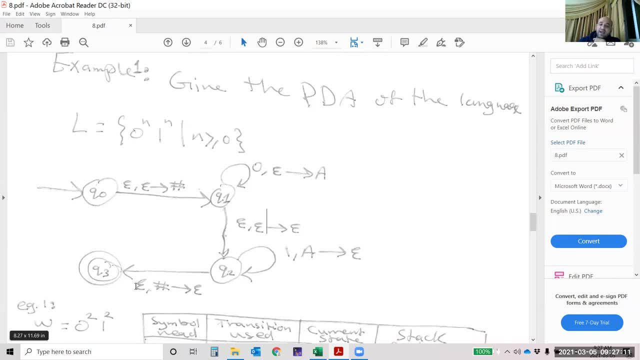 So the thing is A: If I reach to the hash, I have epsilon as an input and I have a hash at the end of the stack- I'll pop the hash and leave its epsilon, which is empty stack then accept. 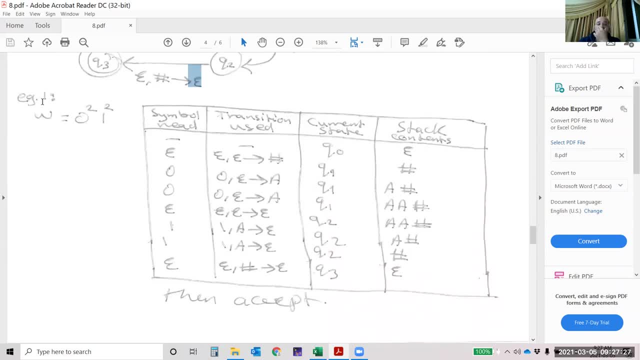 So let's think about this example. If we have some example, like if I give you a string that's saying 0.. 0 to the power 2, 1 to the power 2.. Does this PDA accept this string? 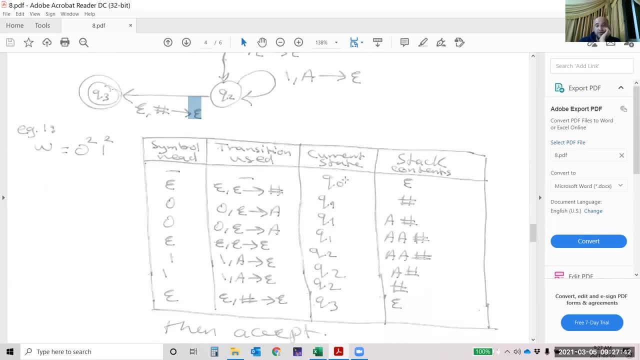 We will see At the beginning nothing. We are at a Q node and the stack contents are epsilon, which is empty. Then I'll use epsilon as an input, Then I'll do an epsilon transition to push the hash and I'll move to Q1 here. 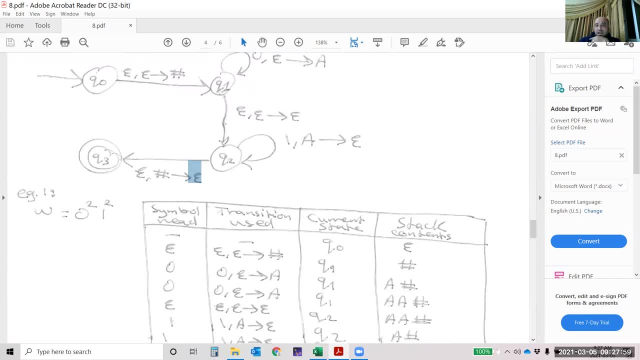 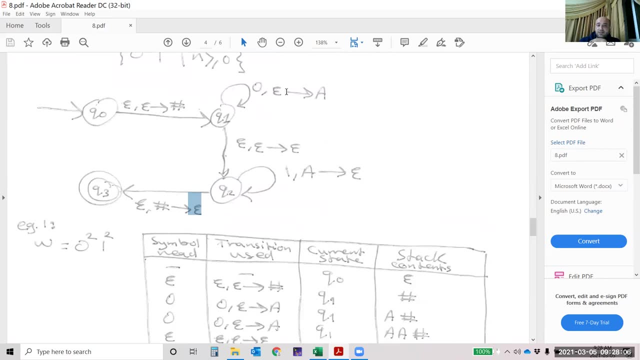 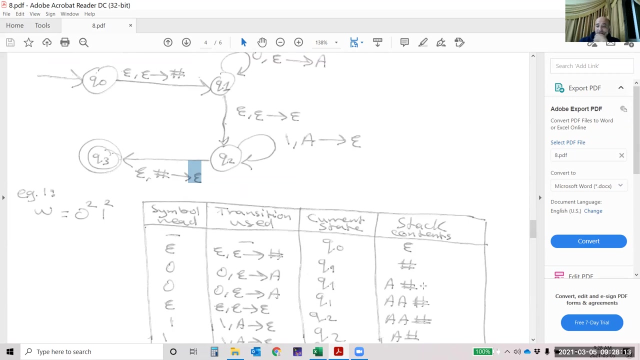 You see epsilon, epsilon hash. I'll move to Q1 here. Then I will read the first 0.. The first 0 saying 0 with epsilon push A and I stay at Q1.. Then the stack content will be A hash. 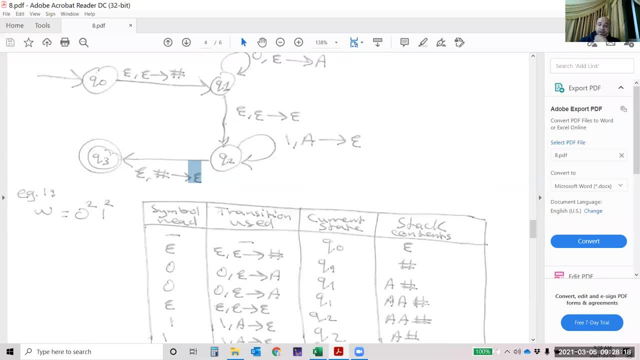 Then I will read the second 0. I'll do the same, Then I'll push A, A hash, Then I'm done with 0s. I'll use epsilon transition to move to the next state And I'm at Q2 that time. 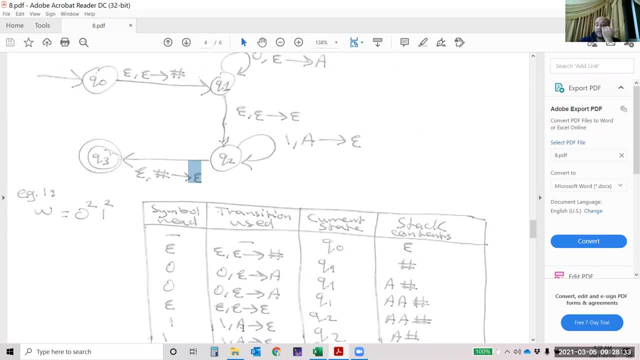 And I will read the first one. I'll pop out an A, You see, after the arrow, which means push, before the arrow means pop, Because sometimes the students are confused when they solve a question. After the arrow means push, before the arrow means pop. 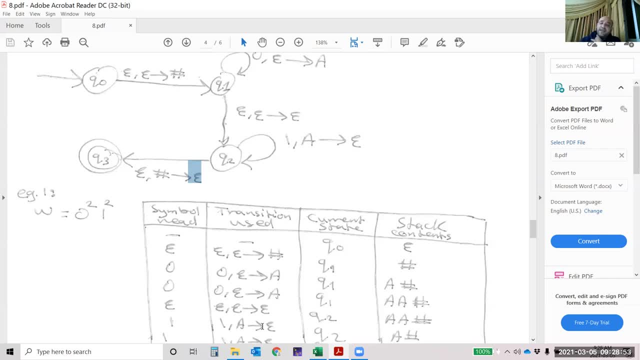 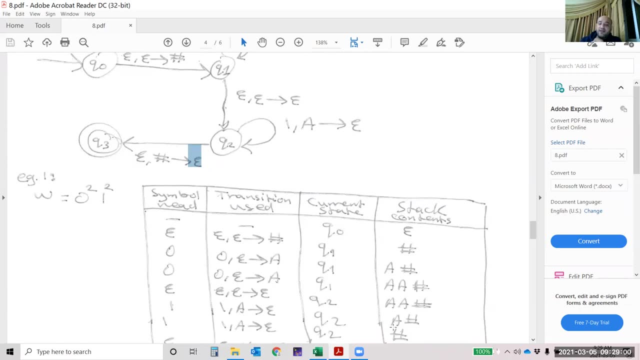 Remember it's like this: Okay, So 1A- epsilon- I'm still at Q2, but the stack content is A, because I put 1A- A1.. Then I read the second one And I put the second. 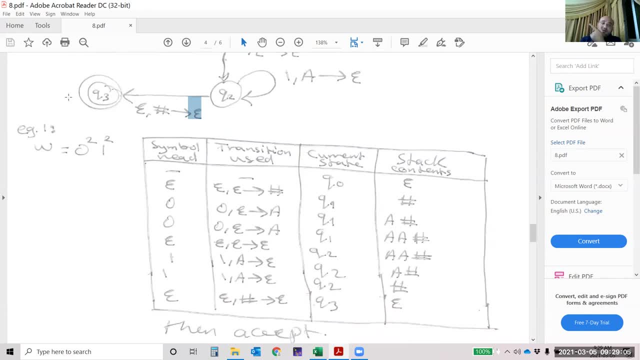 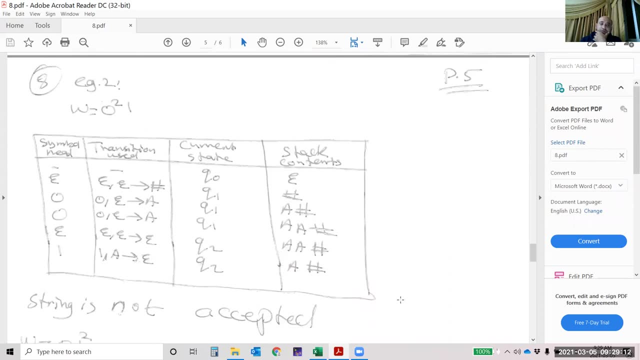 And I'm at hash. Once I read hash, that means move me to Q3 and accept the string. If we take another example which will not be accepted: If I took 021, then I read epsilon, I push the hash. 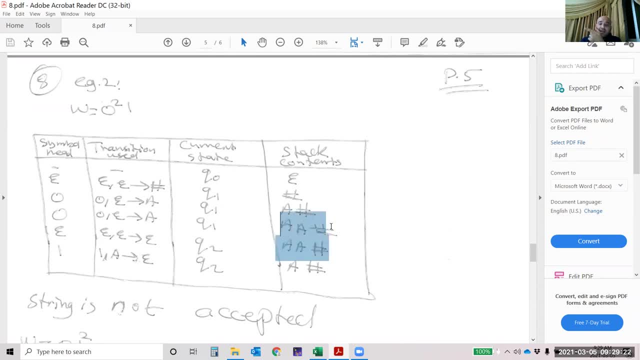 Then I read the first 0,, the second 0. Then the stack content will be A A hash. Then I read an epsilon and move to the one part. I read 1.. I push 1A, Then the stack content is: 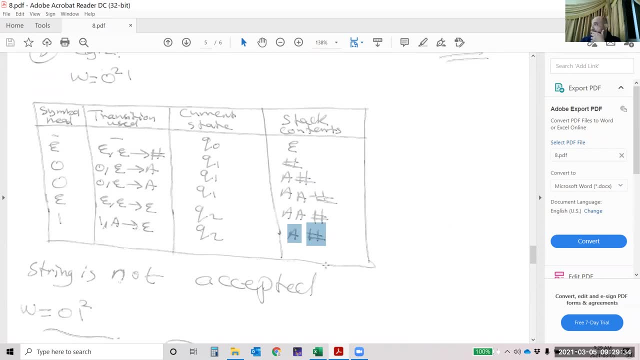 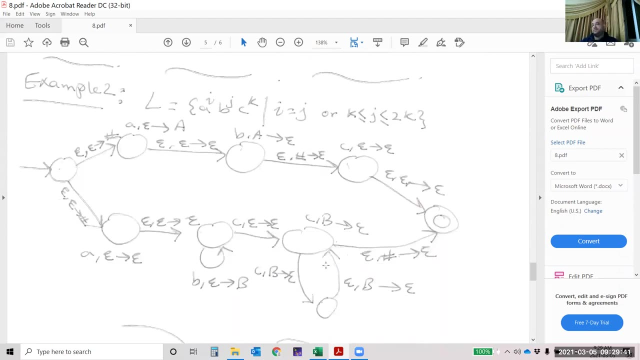 At that time I will stack and the string will not be accepted. Okay, Let's have a more sophisticated example to make sure that we cover the parts of push-down automaton. Now assume that we have the language L, which consists of three symbols: A, B and C. 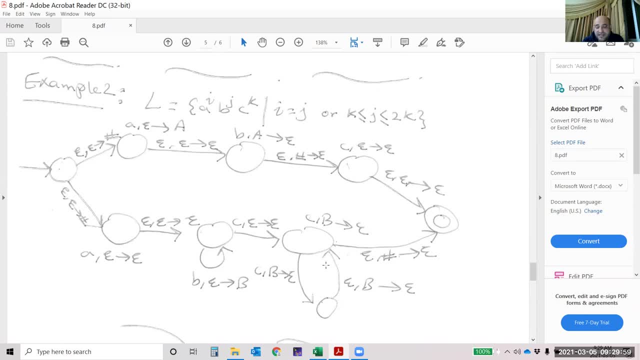 And the power of A is I, B to the power J, C to the power K. And I have here two scenarios to accept. If I equal J, which means if the number of A's equal the number of B's, then accept. 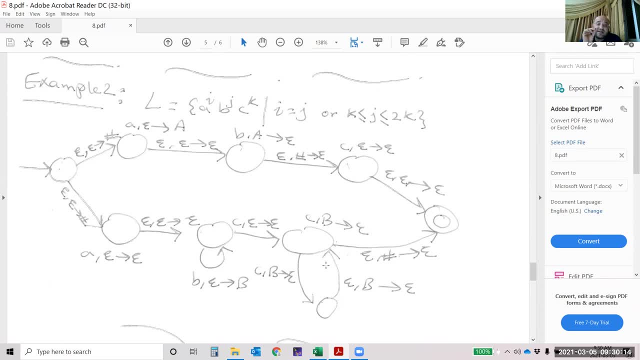 Or the number of B's should be equal to the number of C's, or double the C's Make it a bit complex. So I have here two options: Either I will check the number of A's and B's, I don't care about the number. 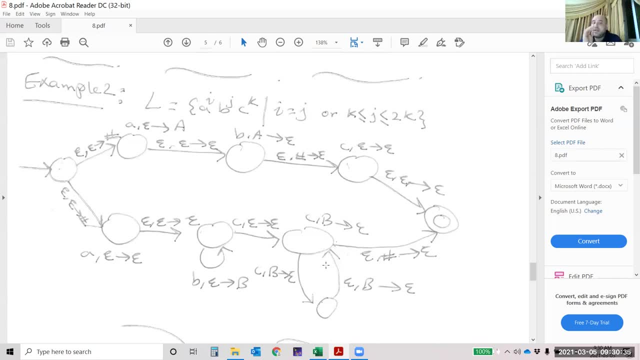 I will check the number of C's. whatever the K is, I would accept. Or if this is not the case, then I have another case: that I will check the B's and C's And the number of C's should be as minimum equal to the number of C's or as maximum, double the number of C's or in between. 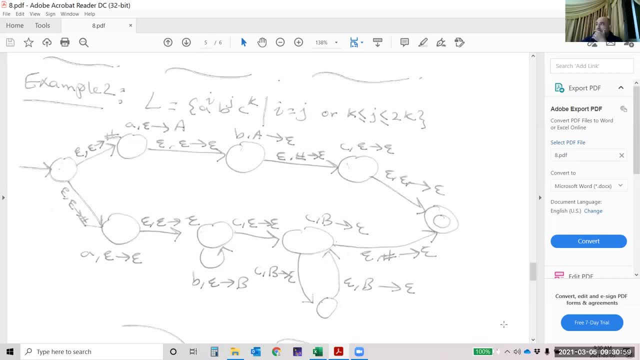 So Okay. So At the beginning, during the non-determinism characteristic of the push-down automata, I could start from the initial state and go into two branches. And we see in NFA we go different ways. So with epsilon transition, either I took this route or that route. we will decide. 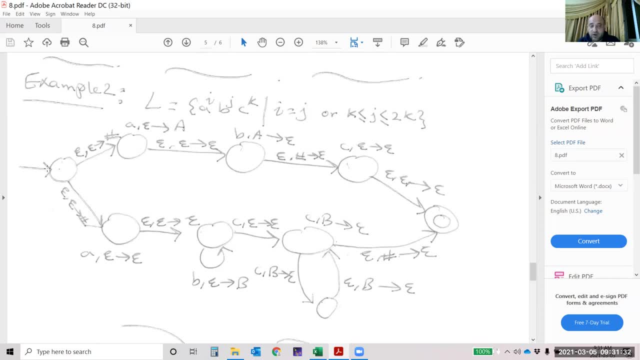 We will push the hash to the stack, which is the initial state, Or initial step. Then I will read the A's And at each time I'm reading the A, which will be the same as 0 to the power n, 1 to the power n, because they are equal. 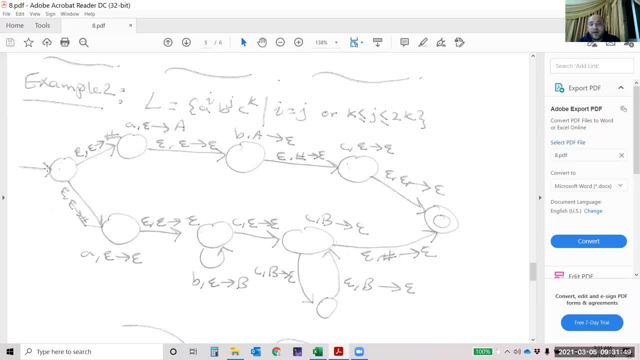 And this is what I'm caring about. So at that time I will read the A's. Each time I read A small, I'll push an A to the stack. Then the next step when I'm reading the B. 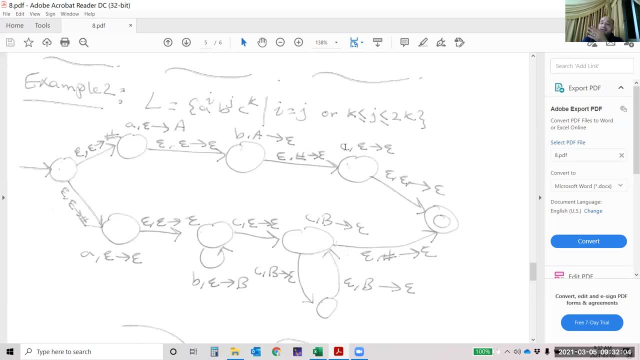 I'll pop an A And once we reach to the hash, whatever we read the C, do nothing And accept. This is the first scenario. The second scenario, which is the other condition here I'll do: I will read A's, because they don't care about A's. 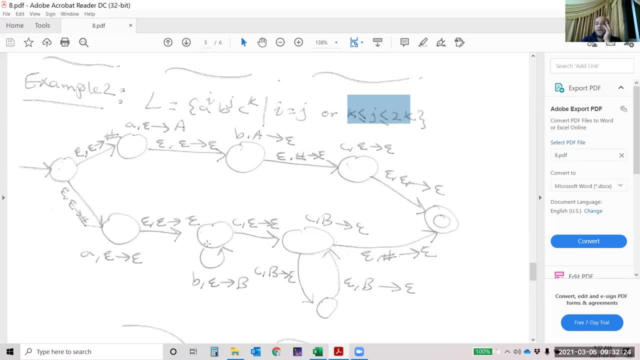 And I will do nothing. Then the issue with B's and C's. And here I have two scenarios, Either with E's Or with C. I'll pop two B's or one B, because you see, the number of C's are in-between. 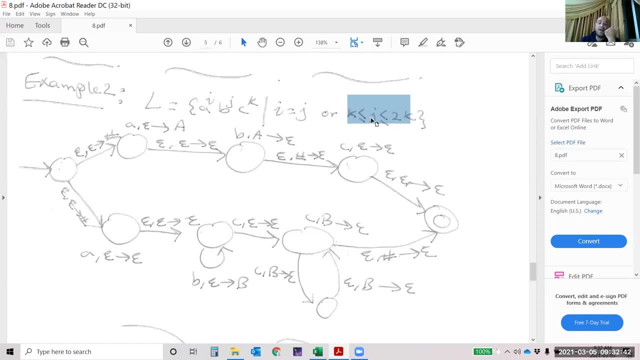 Could be this, could be that or in-between. So how we will decide how to pop one or two. So here we have another scenario we have to follow. So once we read the B, we'll push a B. 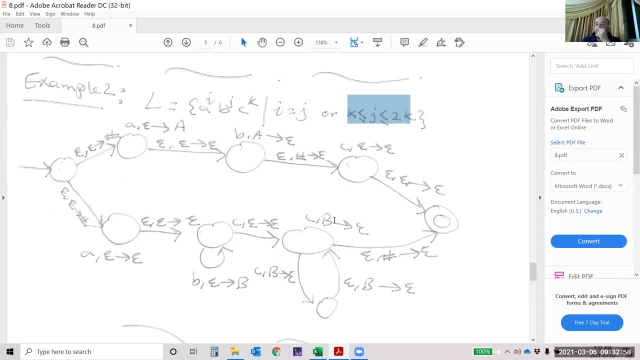 Then, when we read the C, we'll push a B, which is one, Or if I want To pop two B's, I'll go this way: I'll pop B, Then when I back, I'll pop another B. 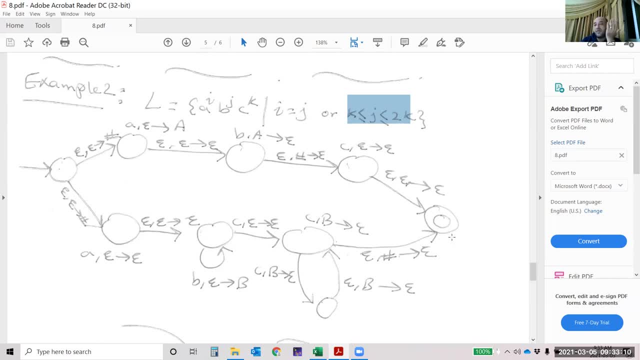 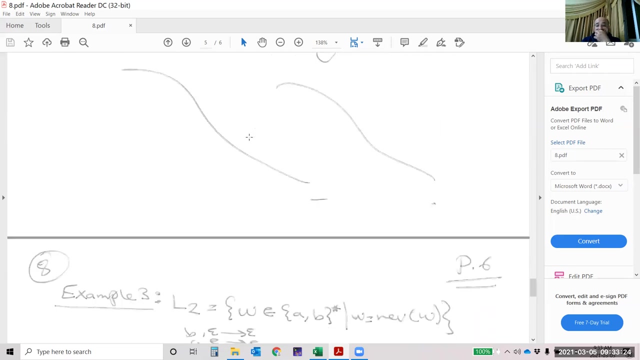 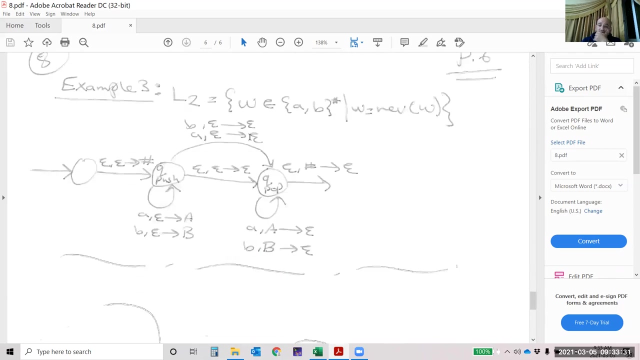 Once we are done and we reach to the hash, we'll go to the accept state. Is that clear guys? This is the push-down automata for this language. Clear Questions Before moving to example three. Okay, With example three. 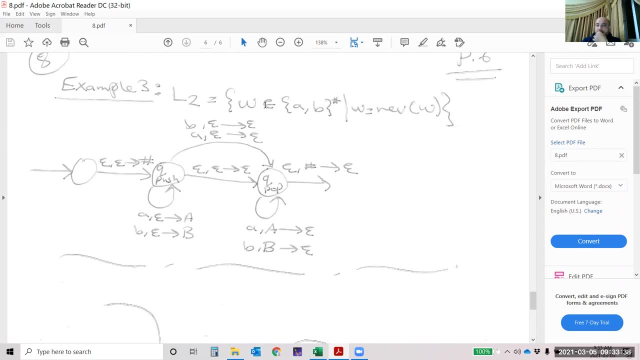 Assume that L2, a language that consists of a string, W, W belongs to A B star, where W is the reverse of W. Okay, you will ask me here a question: When I will start to push, then when I will do the pop. 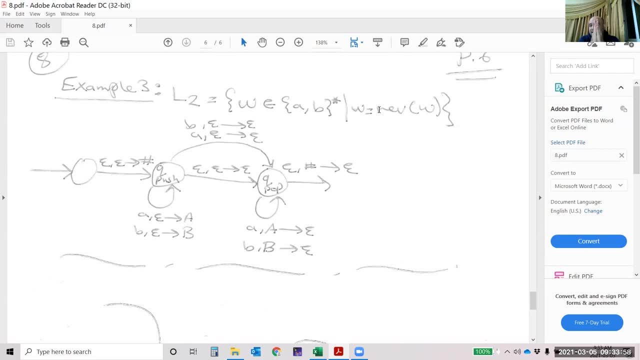 The thing here is at the center or the middle point of the string. if it's even or odd, it will be different. If it's even the middle two symbols, I will do nothing for them. But if it's odd, 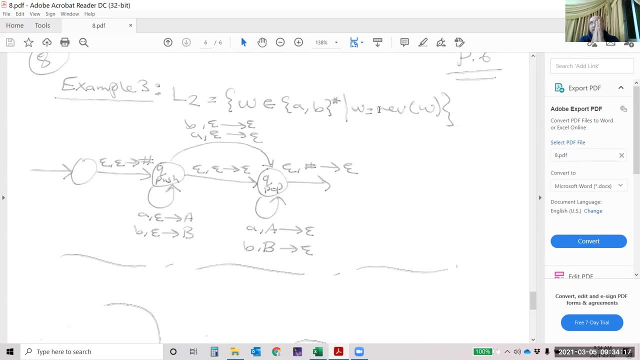 I will keep just leave that middle. For example, if I have a string A, B, B, B, A, So the second B is in the middle, But if I have A, B, A, B, A, B, the middle A, B will be the middle of the string. 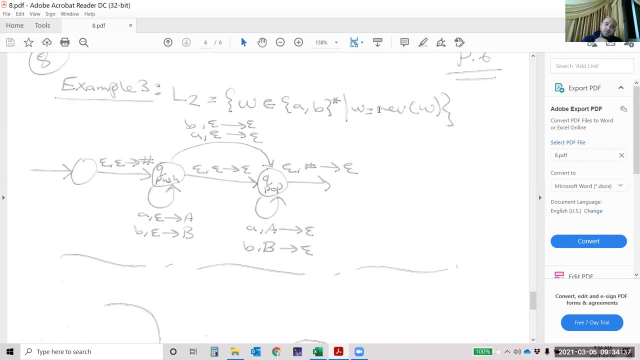 So I'll take both scenarios. We will push the hash And we have two states: Q push and Q pop, Q push A's. And if I read B push, B. Once I'm done, either I'll go to start popping them. 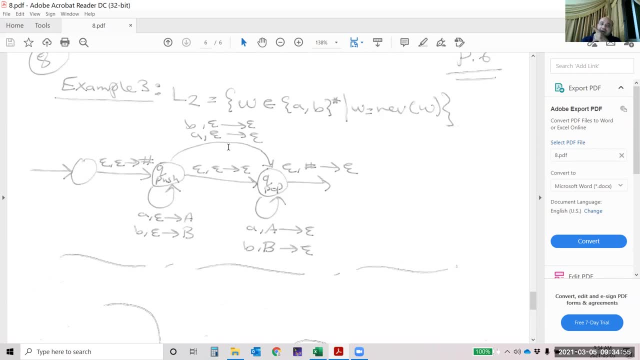 to reverse the string And if, at the middle point, if there is the middle point is B do nothing or A do nothing Or both, take them both, Then move to the transition and at that time we are reversing the string. 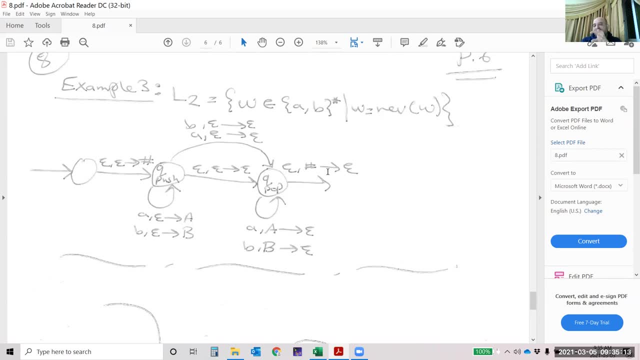 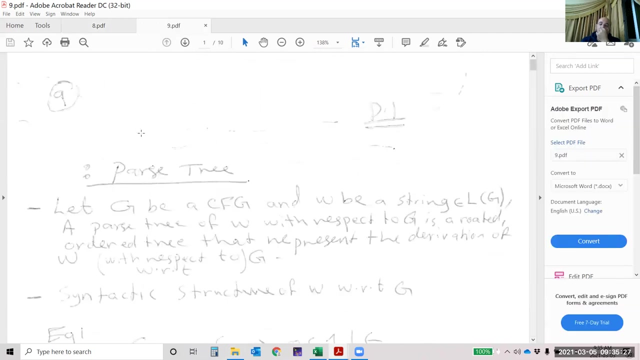 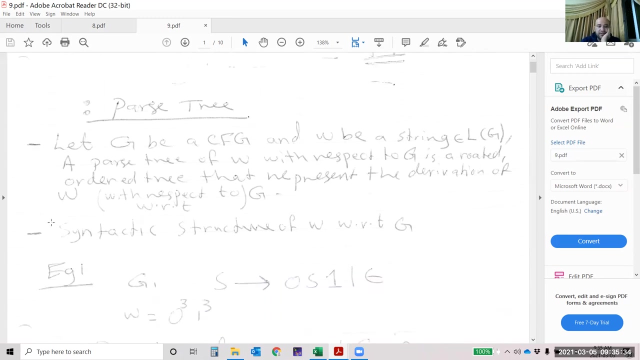 Clear. So normally when you have a question, consider different scenarios. Clear guys: Okay. So let's go to nine. Okay, We talk in the second part of the handout about the parse tree. It is a simple topic, but we will talk about it again. 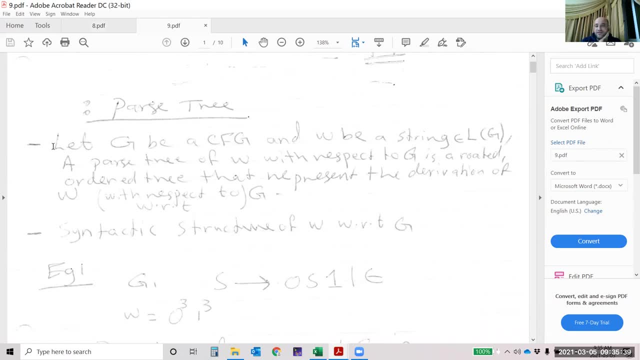 Let G be a CFG context-free grammar And we W is a string that belongs to that grammar. A parse tree of W with respect to G is rooted order tree. What do we mean? Rooted order tree? We will see how that. 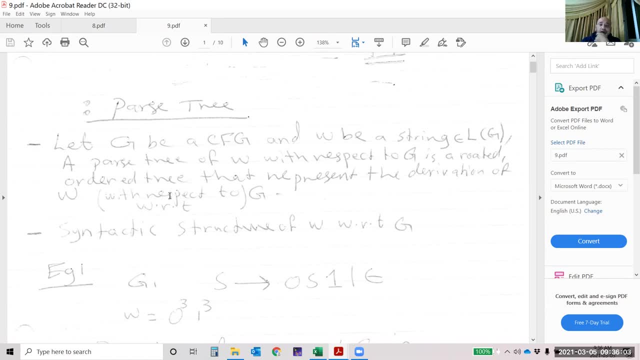 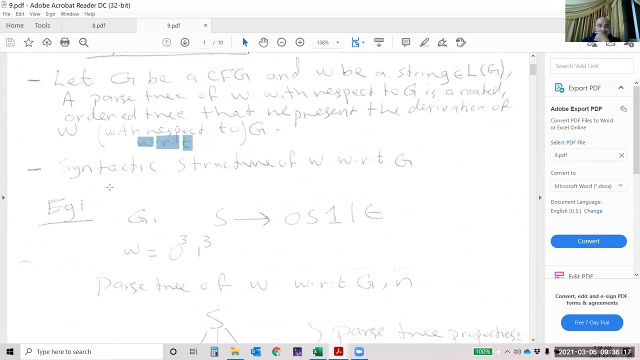 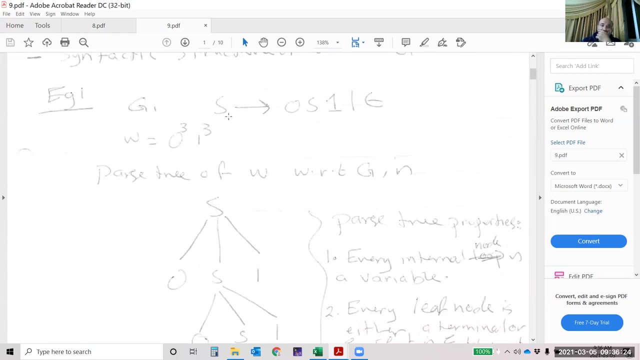 That represent the derivation of W with respect to G And with respect, we will use WRT from now. So example: If we have the grammar G, which take the first, the example that we took, which is 0S1.. 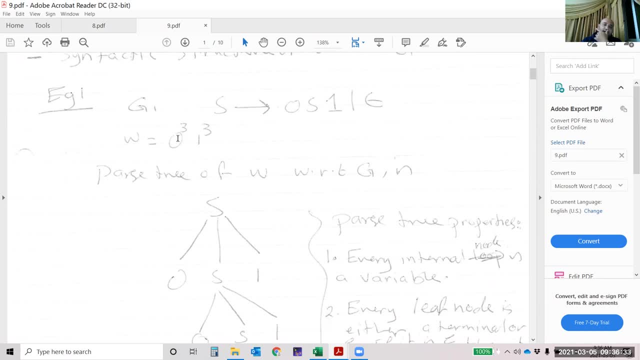 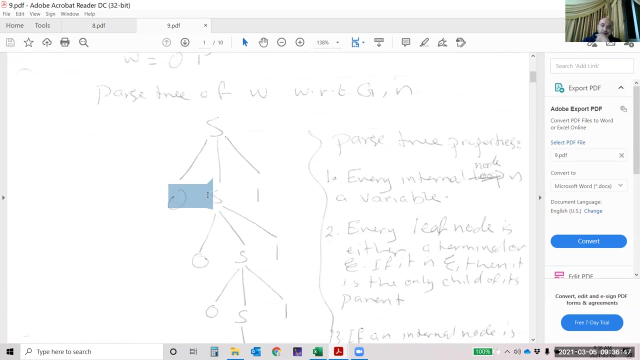 And we have O to the power or epsilon, O to the power 3 and 1 to, or 0 to the power 3 and 1 to the power 3.. Parse tree of W. with respect to that grammar is: S will be replaced with 0S1.. 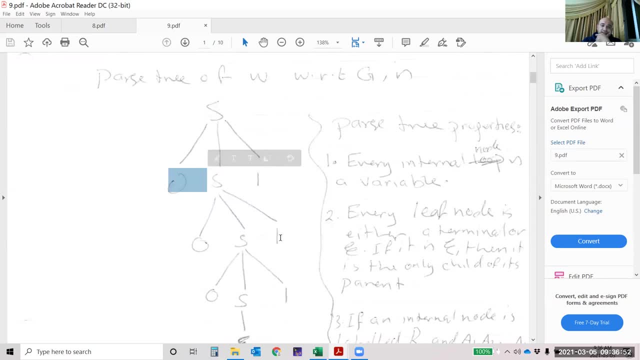 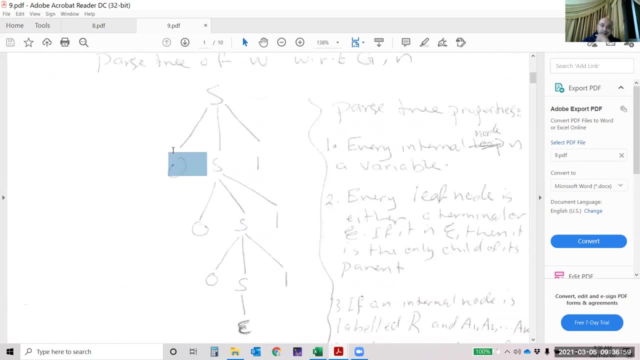 Then we have a 3 here, Then 0S1.. Then 0S1.. At that time I have three 0s and three 1s. Then we'll go to the epsilon. So every internal node is a variable. 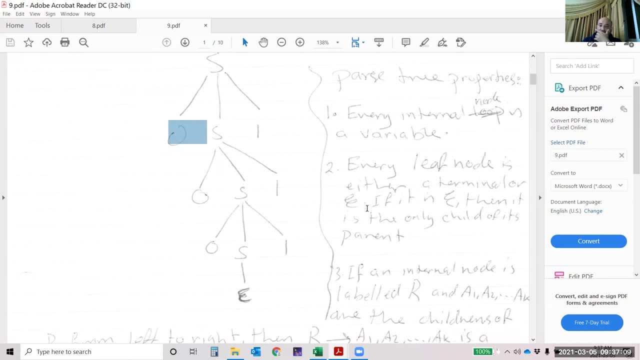 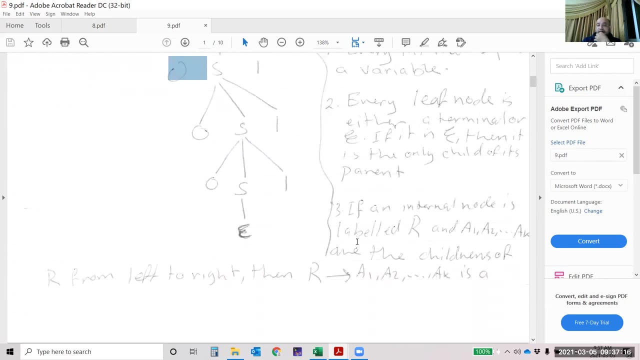 Every leave node is either a terminal or epsilon. If it's epsilon, then it is only child of its parent. If an internal node labeled R And if an internal node labeled R And if an internal node labeled R, Then 0S1 to AK are the childest of R, from the left to right then R. 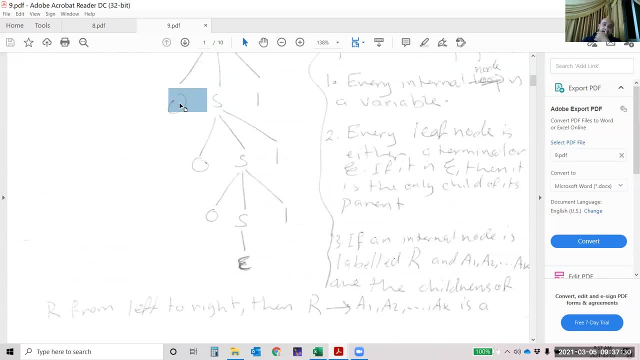 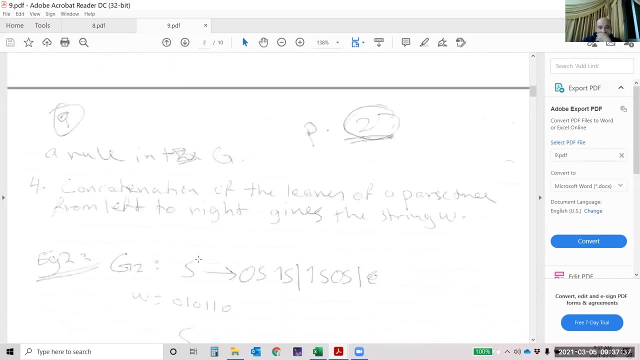 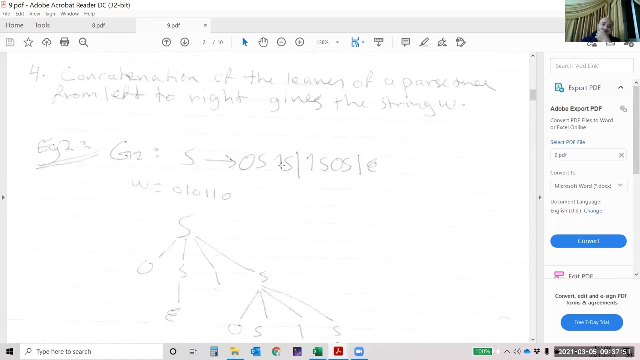 So how we will read it: 0, 0, 0 from left to right. Concentration of the leaves of a parse tree. from left to right gives the string W. Now example two: if we have 0S1S or 1S0S. our second example yesterday. 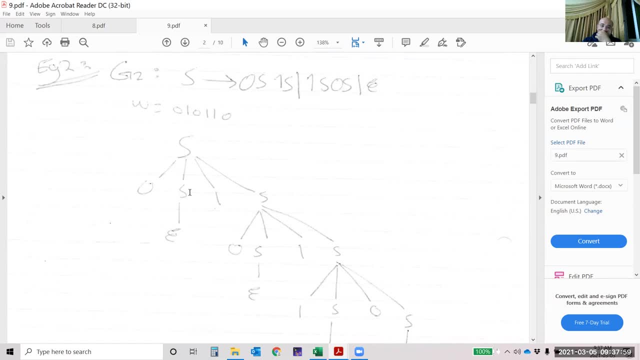 So here we have S, which will replace it with 0S1S, And the first S we will replace it with epsilon. Then, because we have this string, Then we have 0, 1 now from the left. 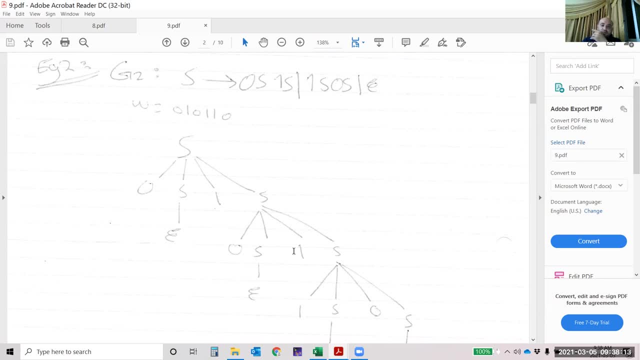 Then we will replace S with 0S1S. This one will be epsilon, Then it will be 0, 1,, 0, 1.. And here we have the other one, which is 1S0S, And we replace those with epsilon. 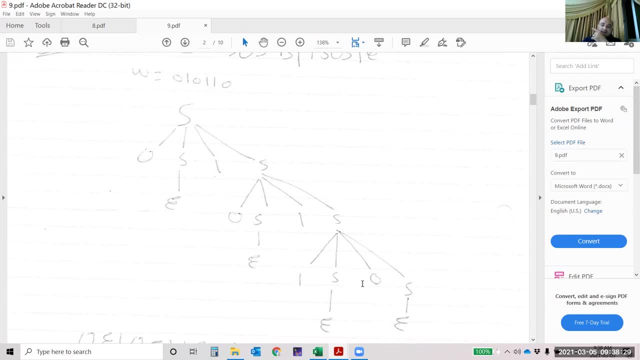 So we read it: 0, 1, 0, 1, 1, 0, 1.. Which is our string. You see how we read it From left to right. So you see here: 0, epsilon, 1, 0.. 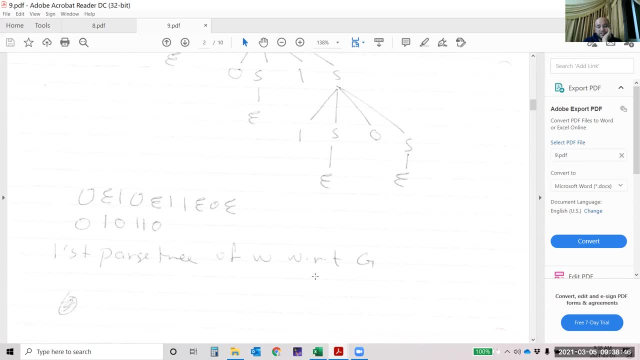 It's a parse tree of W with respect to G. This is the second parse tree with respect to G. We can do it this way, So you can do it whatever you want. We can have multiple parse trees for some string, So some string it might be different in the parse tree. 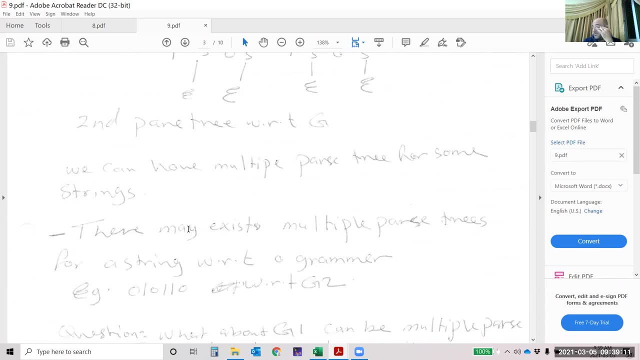 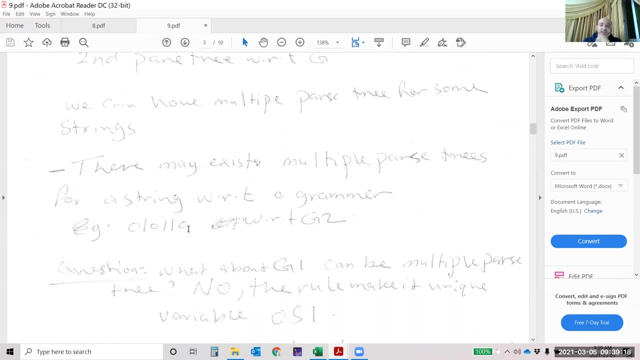 However, if it's Let me arrive to the accepted state, then we are okay. There are many. exist multiple parse trees for a string with respect to a grammar Like 0, 1, 0, 1, 1, 0.. 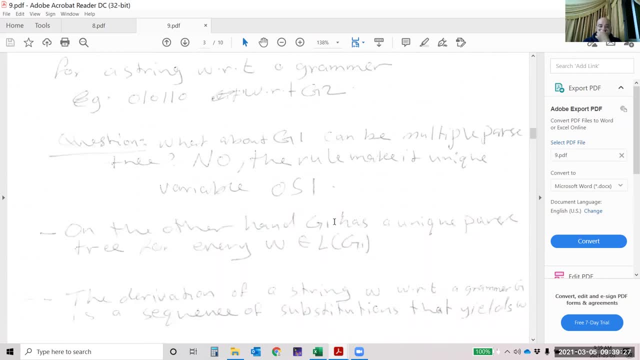 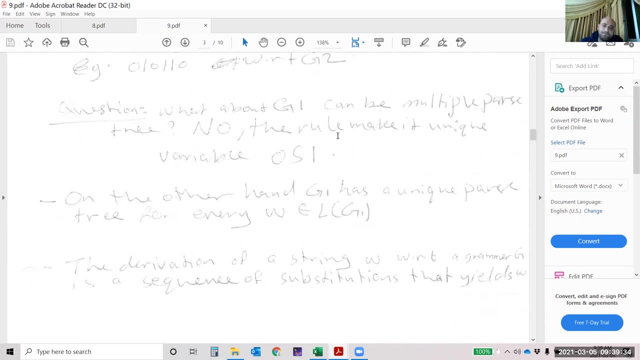 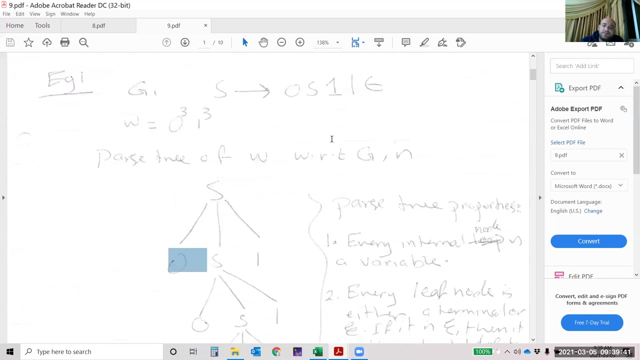 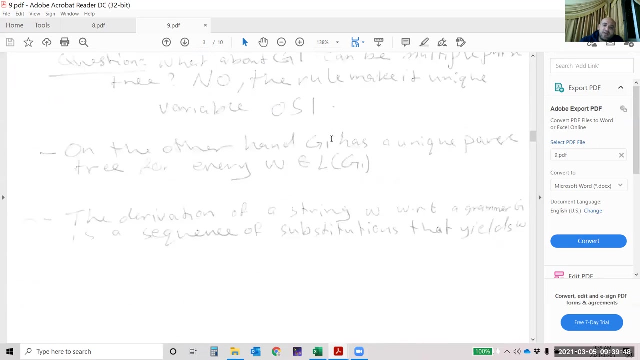 With respect to G2 also, it is accepted. Question: What about G1? can be multiple parse tree? This one I'm asking here, This is G1.. No, We cannot have multiple, But the other example show you that we might. 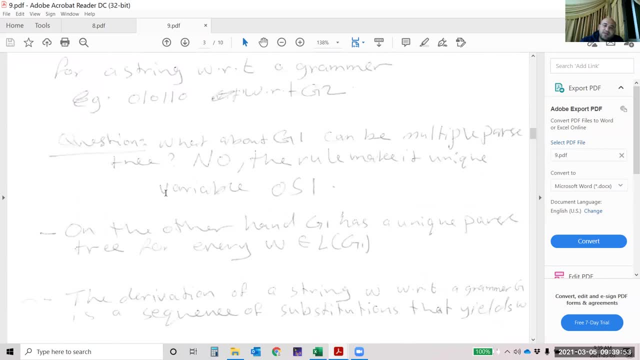 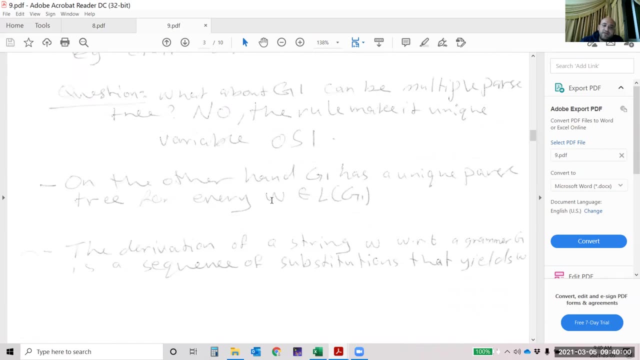 Sometimes we have. So let's make unique variable 0 as 1.. On the other hand, G1 has a unique parse tree, for every W belongs to L in G1.. The derivation of a string with respect to a grammar G is a sequence of a substitution that yields W. 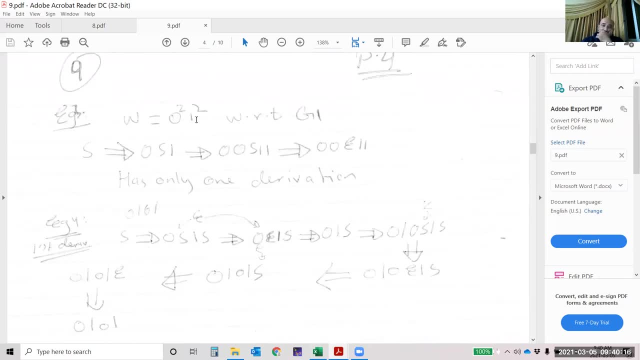 So if we have W O square, 1 square with respect to G1, then we'll have 0, S1, 0, 0, S1, 1, 0, 0, epsilon 1, 1 has only one derivation. 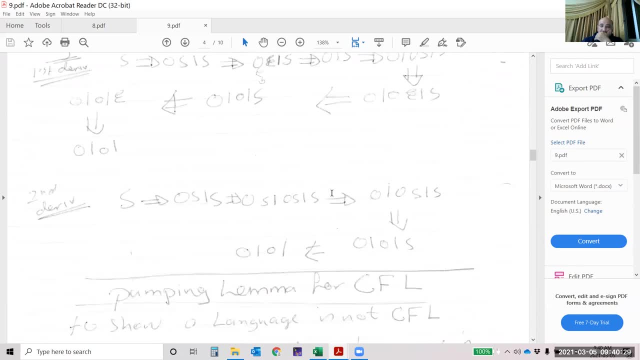 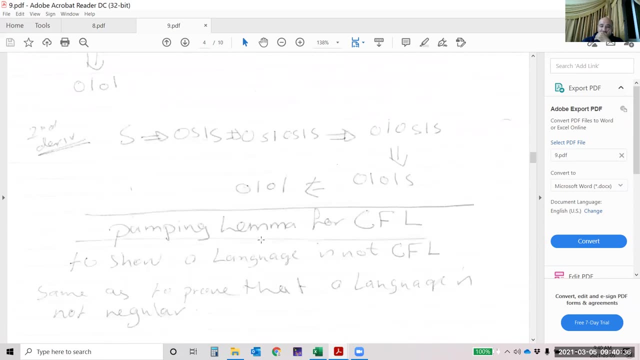 Second derivation: 0, S1, S 0, S1, S 0, S1, S S, and it will represent this one. Now we'll come to your friend pumping lemma for CFO Guys. the same concept. 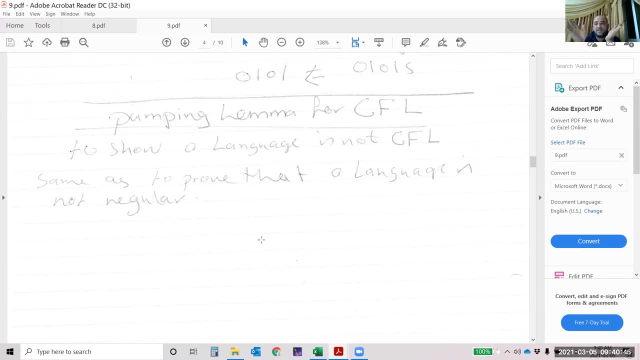 But now with five simple. We split the string to five simple: U, V, X Y Z. Before we use X Y Z. It's the same concept, But here we'll add the power to the. 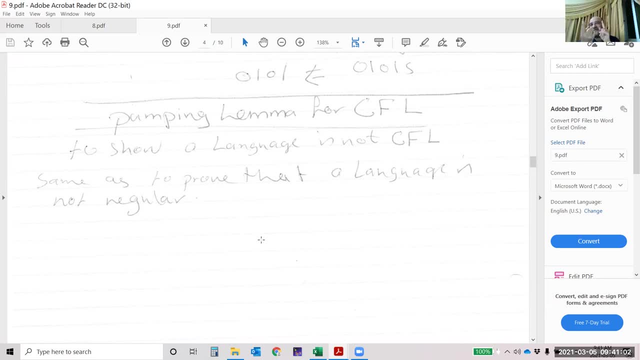 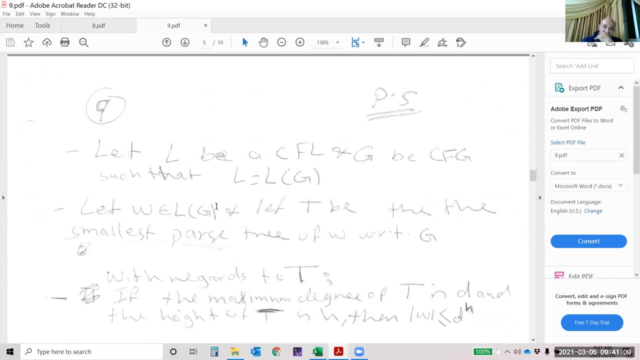 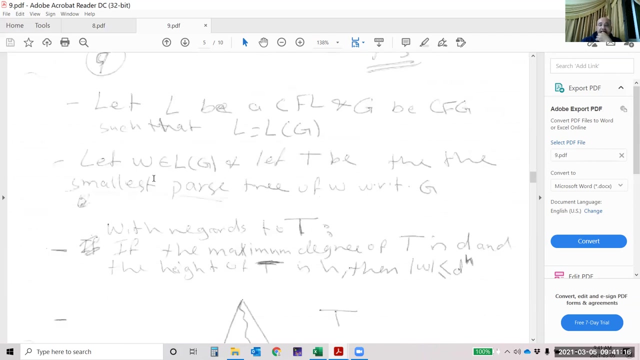 V and Y, Or if you use V, U, it will be for the U and the Y. Now let L be a context free grammar And G be a CFG, such that L equal L of G, Let W belong to L of G and let T be the smallest parses tree of W with respect to G. 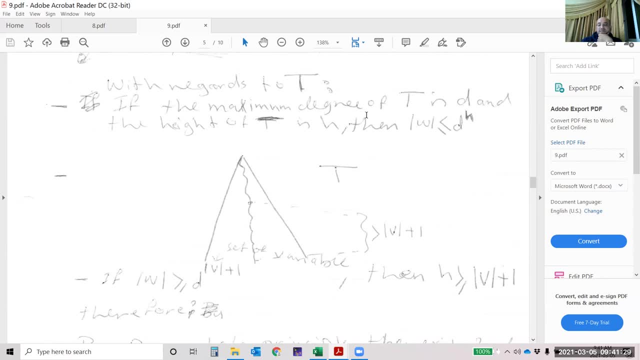 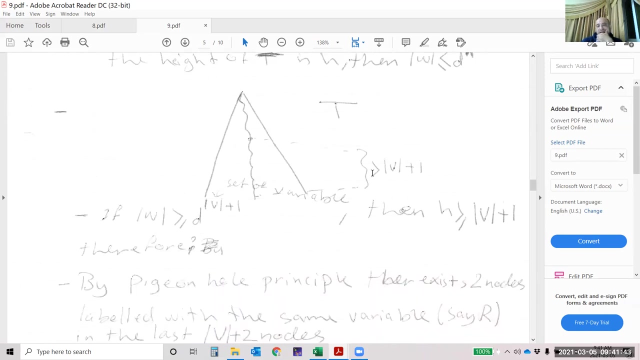 With regard to T, if the maximum degree of T is D and the height of T is H, then the length of W is less or equal D to the power H. So this is the parsed tree of T, And here we have the height. 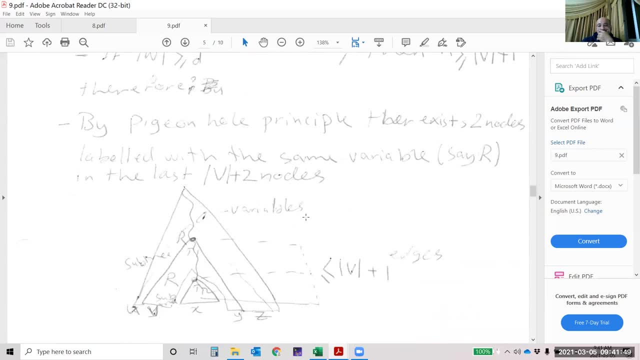 And we use these things By Pigeon-Hall principle. there exists two nodes labeled with the same variable, Say R. Here We have R and R In the last V plus two nodes. So here X, V, X, Y. 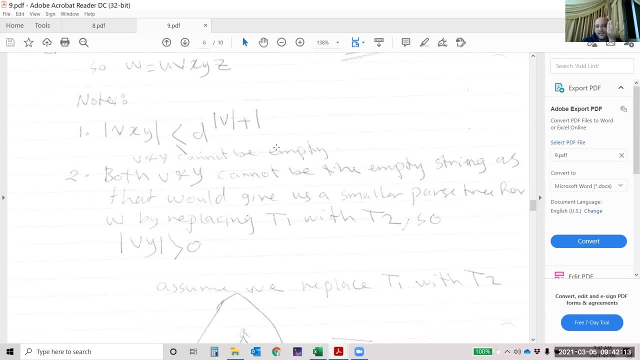 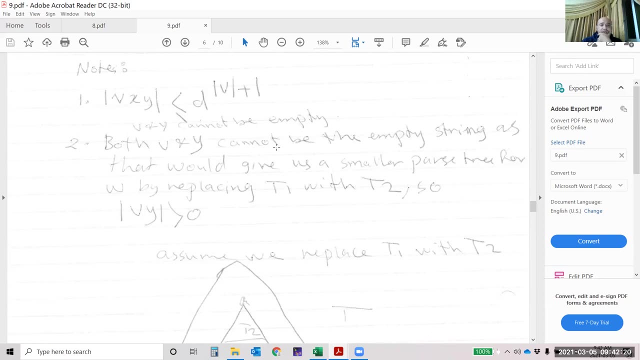 X, Y less than D. You know we don't need this proof, I just write it for you to understand how we come out with Pigeon-Hall principle: Both V and Y cannot be the empty string. V and Y cannot be the empty string. 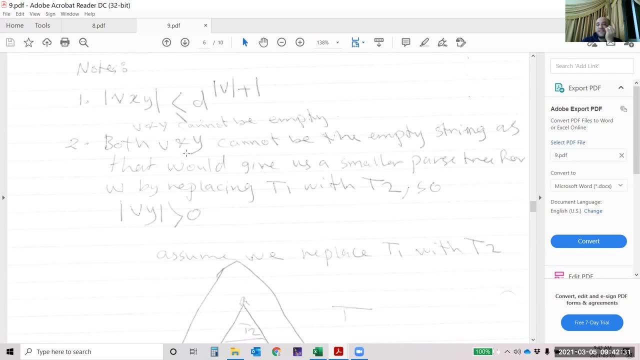 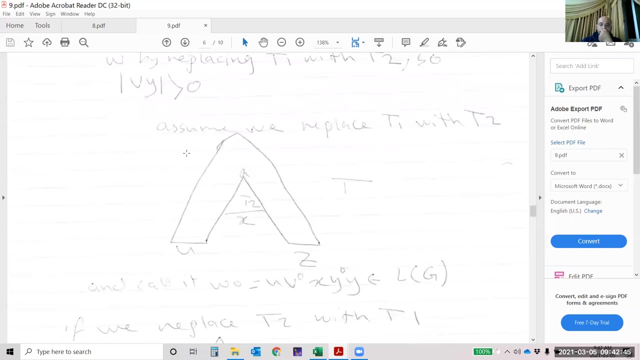 Same as in non-regular languages. we said: Y cannot be an empty string, X could be, Z could be, But Y no. Here Context-free grammar. We have two strings that should not be empty: V and Y. And here are the derivation: 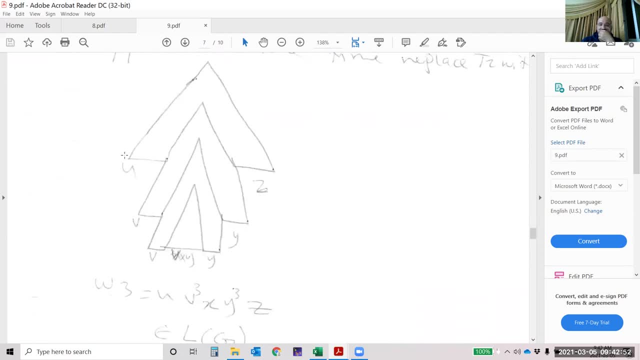 I'm not going to read that. We'll start solving Here: U V, V, V Y Y Y Z V, X Y, So U V, 3. X Y, 3, Z. 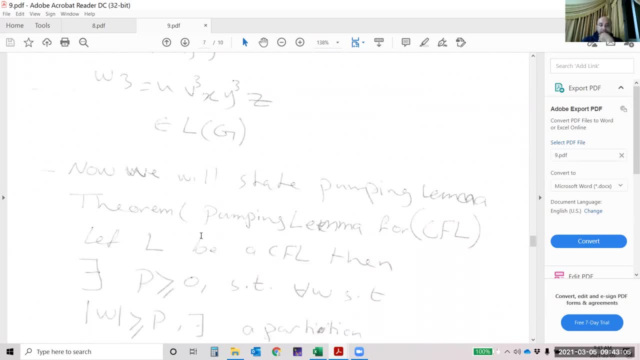 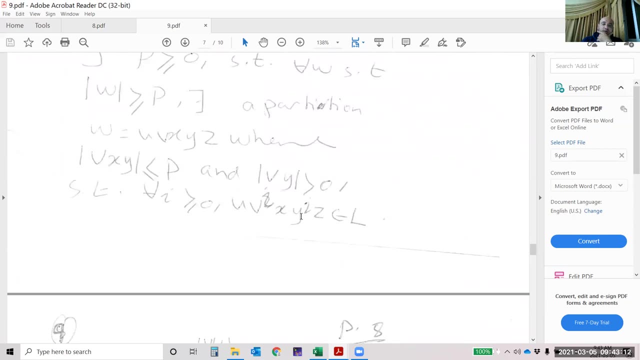 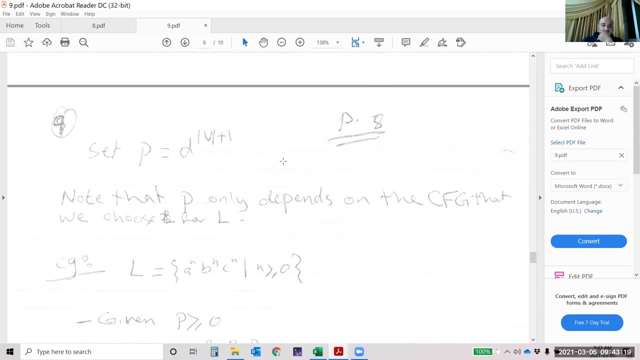 Belong to L of G. Now we will state pumping lemma theorem. Pumping lemma theorem: The same thing as before, But here we have U, V to the power I and Y to the power I should belong to, L And set P equal D to the power V plus 1.. 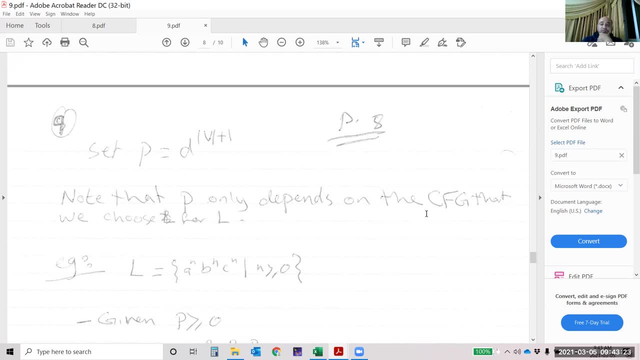 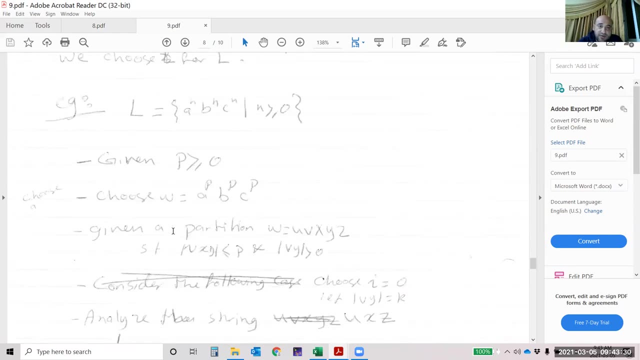 Note that P only depends on the context-free grammar that we choose for L. Now assume this example: If L is A to the power N, B to the power N, C to the power N Given, P greater or equal 0.. 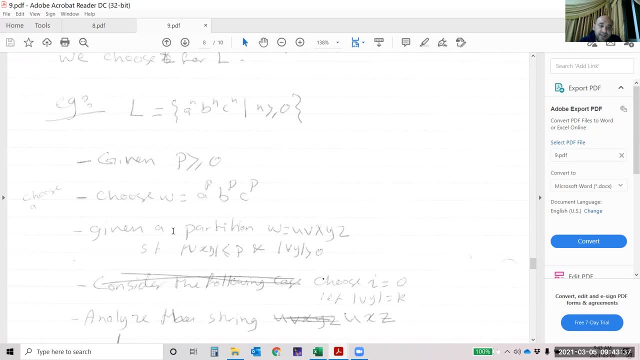 Choose: W equal A to the power P, B to the power P, C to the power P. Given A a portion W U, V X Y Z, Such that V X Y less or equal to P and V Y greater than 0.. 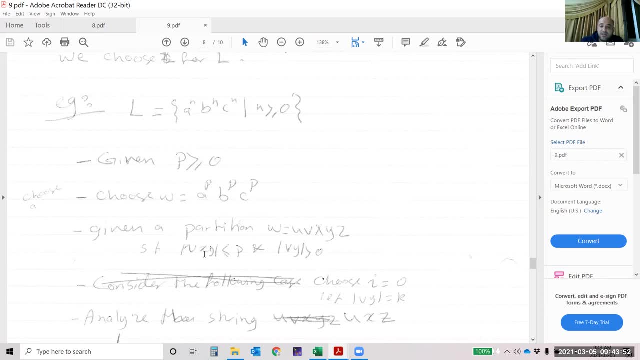 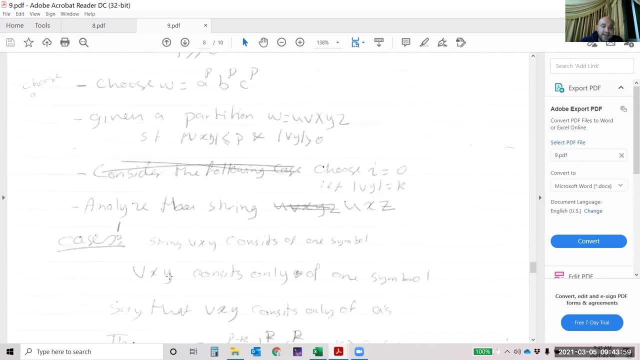 The length of V and Y is greater than 0. Choose: I equal 0.. Let V: Y equal K. Analyze the string U X Z, Case 1.. Now here In our example, In case 1.. 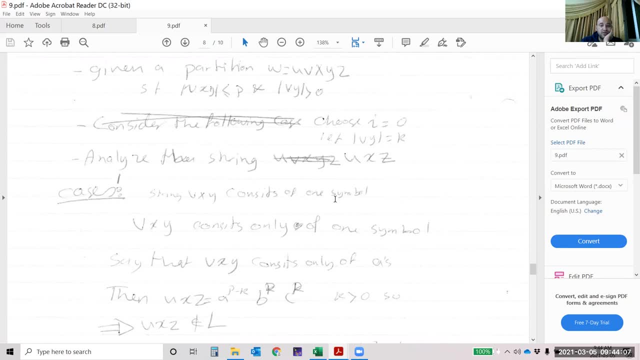 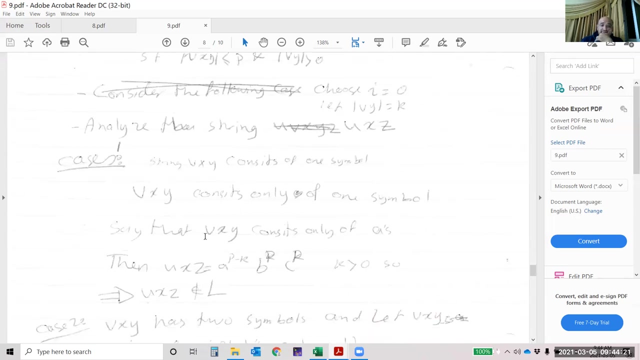 String V X Y Consists of one symbol. V X Y cannot only One symbol, Cannot be- Contains only one symbol. Say that V X Y consists of A's, Then U X equal A to the power P minus K. 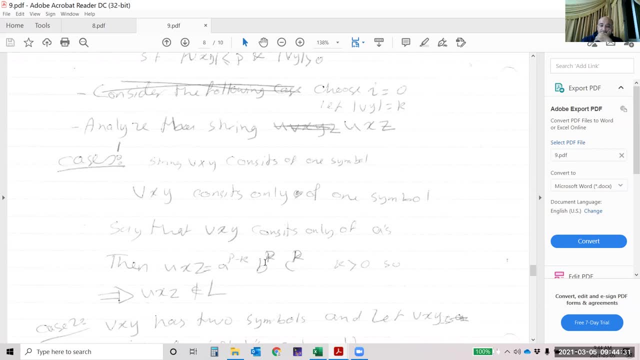 B to the power P and C to the power P Where K is greater than 0. So U X Z is not belonging to us From the beginning Because we have a different power here. They should be the same. 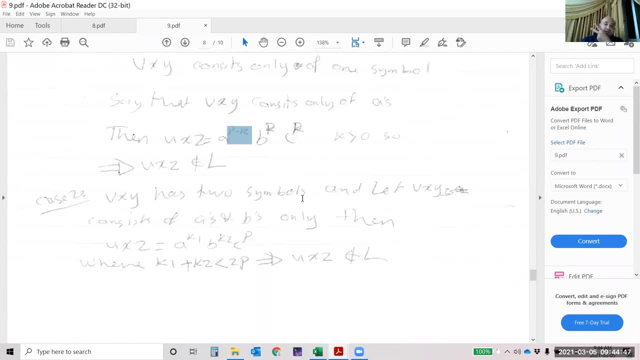 Case 2.. V X Y has two symbols only, And let V X Y consist of A's and B's only. Then U X Z equal. A to the power K1.. B to the power K2.. 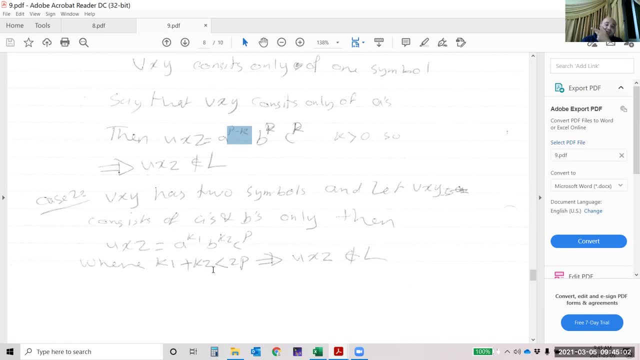 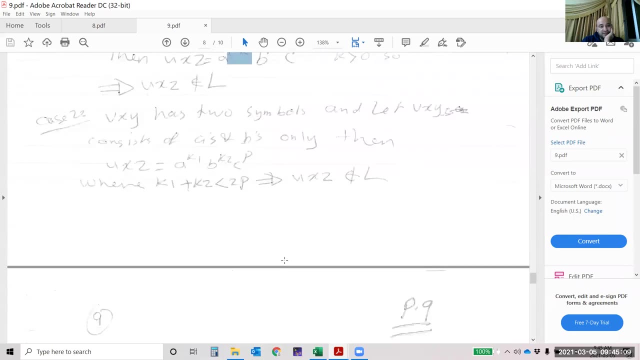 C to the power P. Where K1 and K2 less than 2P, Then U X, Y, Z is not belonging to L. The same principles, guys. V, X, Y cannot contain all three symbols A, B and C. 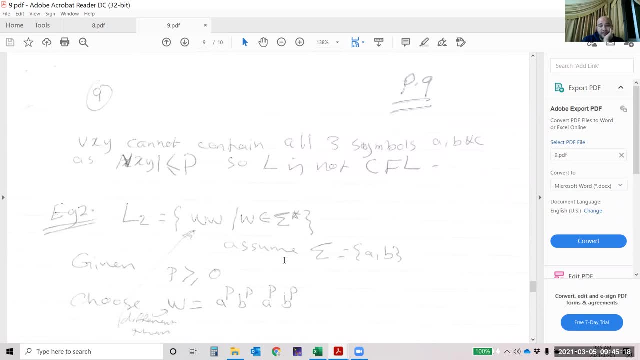 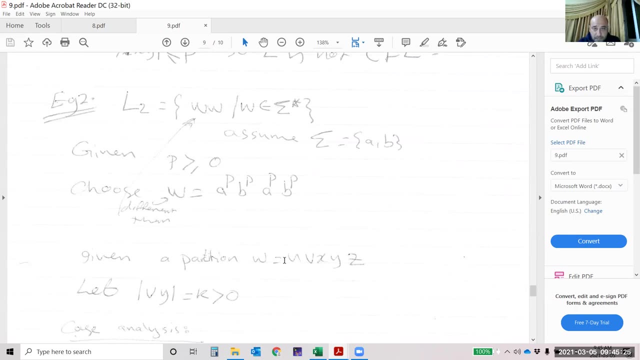 As V, X, Y less than P. So L is not a context-free language. Another example: If we have the string W, W Where W belongs to sigma star, Assume sigma equal A and B. Choose W Equal A to the power B. 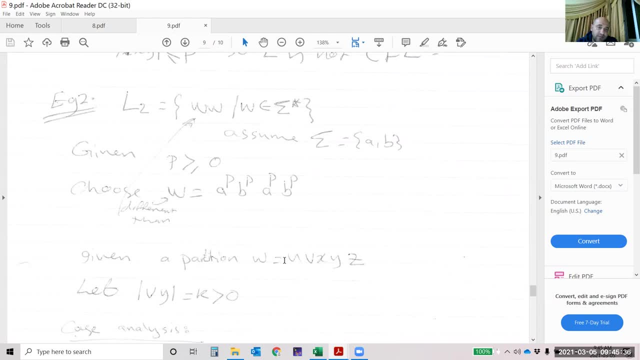 B to the power B And A to the power P, B to the power P, Because we have W, W Given a portion, W, X, U, V, X, Y and Z, Let the length of V? Y equal K and greater than 0.. 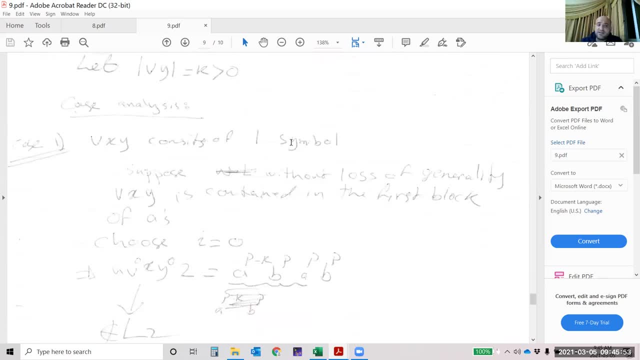 The case analysis. The first case, V X Y, consists of one symbol. Suppose without loss of generality. V X Y is contained in the first block of A's Choose I equals 0.. So U V to the power 0.. 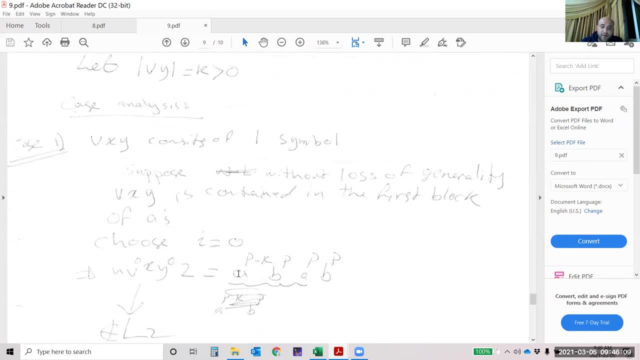 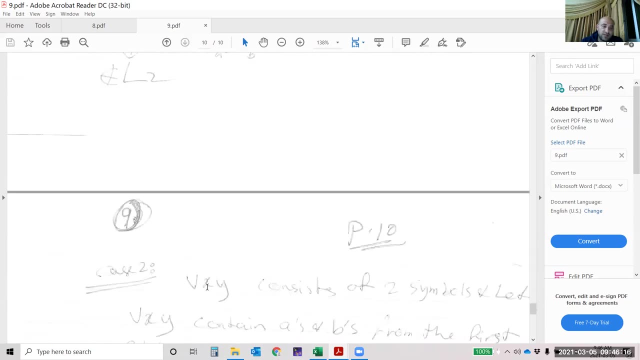 X, Y to the power 0. And Z, Then it will be A to the power P minus K, B to the power P, A to the power P, B to the power P Which does not belong to that length, Case 2.. 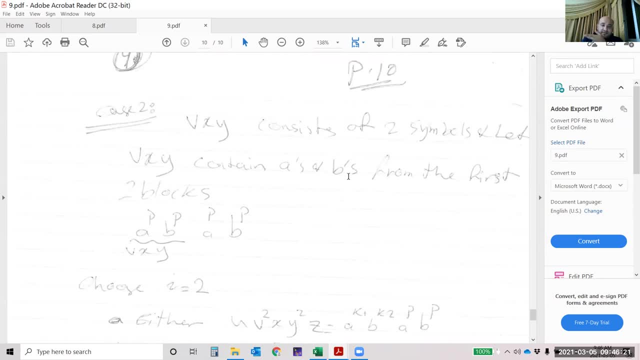 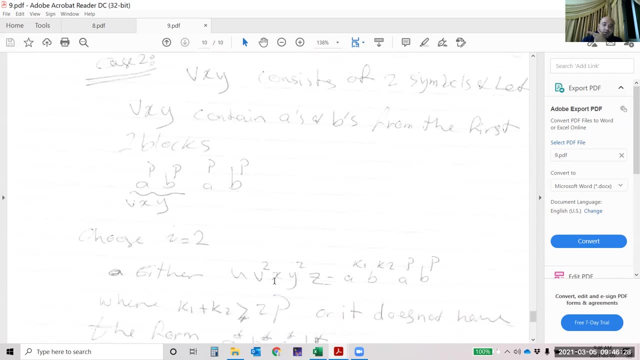 If it consists of two symbols, A's and B's, Then A to the power P, B to the power P, A to the power P, And this is V, X and Y Choose, I equal 2.. So U, V. 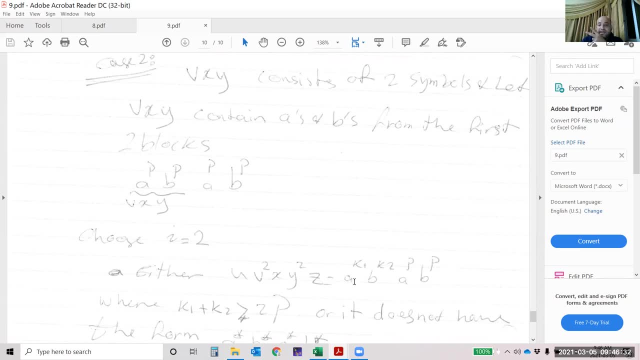 Square X, Y, Square Z Square, Which will be: A to the power K1.. B to the power K2.. A, B, A, P, Where K1 and K2 is greater than 2 P's. 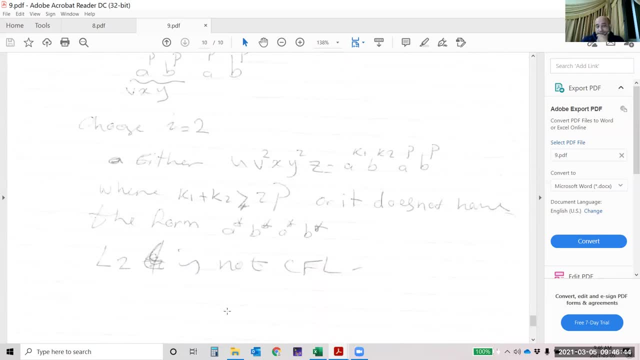 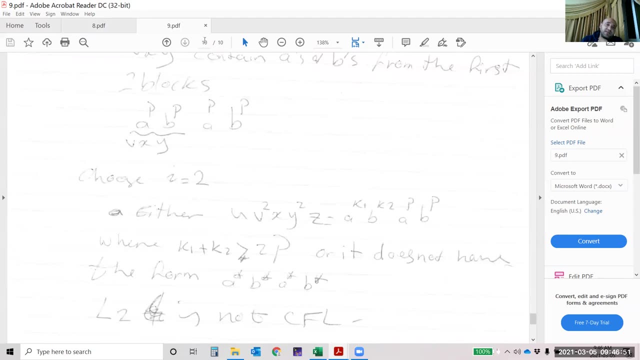 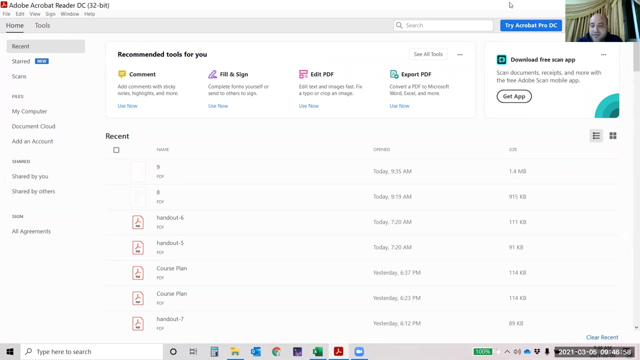 And this is not contained in CFL. Same principles, guys, Same principles. More examples of pumping lemma will be solved in next week's tutorial With the TA. Any questions? Okay, So we will move Turing machines. We will take the handout. 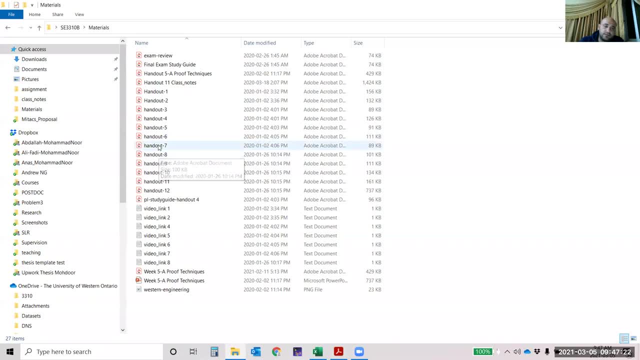 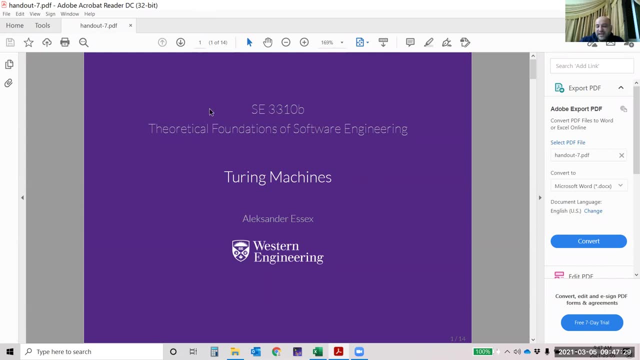 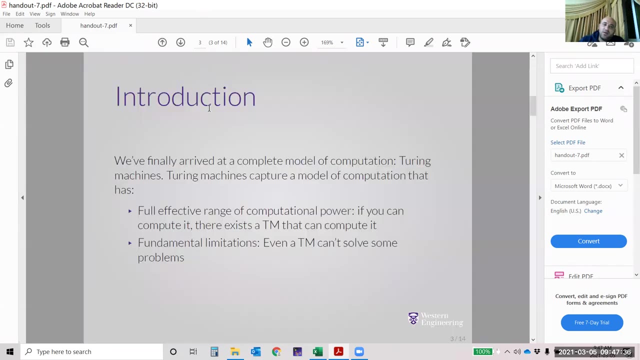 And now we will move to the Turing machines. Okay, next class, we will do the class notes. what is a Turing machine? we have finally arrived at the complete of the model of the computation. this is the last model of computation and graphs and you know context, free grammars and all of these things we finally arrived to at a 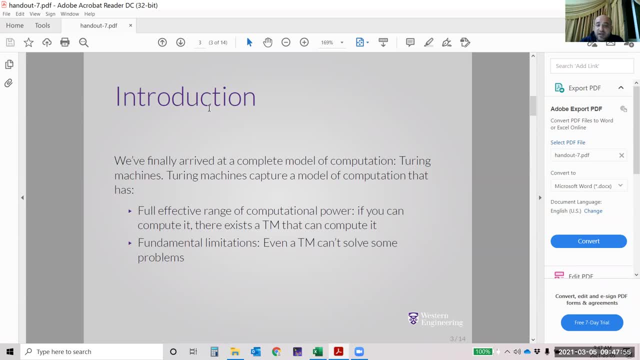 complete model of computation: Turing machine. Turing machine capture a model of computation that has full, effective range of computational power. if you compute it, there is exist a Turing machine that can compute it. fundamental limitations: even a Turing machine cannot solve some problems. even Turing machine, even it's a powerful computational model. however, sometimes there 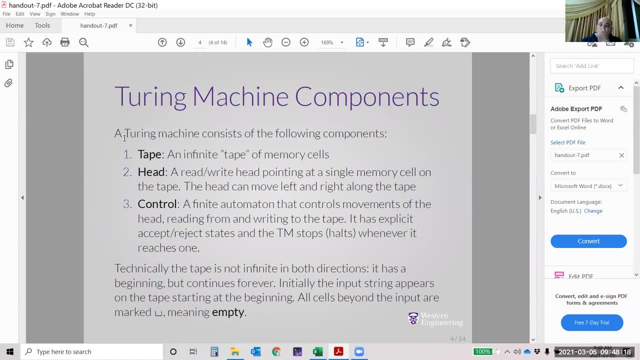 are some problems that could not be computed using Turing machine. so Turing machine consists of the following components: tape, an un-finite tape of memory cells. head to read and write, hit pointing a single memory cell on the tape. the head can move left and right here here in Turing machine. in Turing machine we can. 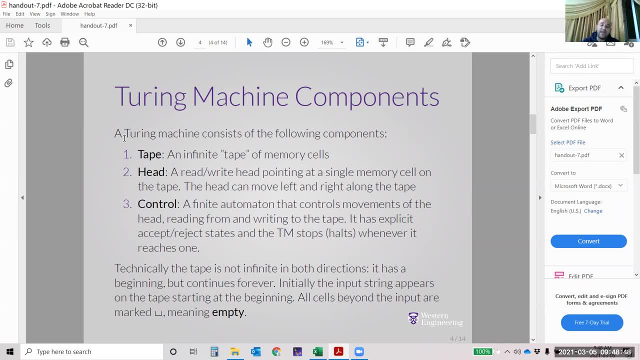 go left and right, not like the stack, we can access only from one direction. control a finite automaton that control movements of the head, reading from and writing onto the tape. it has a explicit accept or reject state and the Turing machine stop, halts, we call it. we never reach one. technically the tape is not infinite in both. 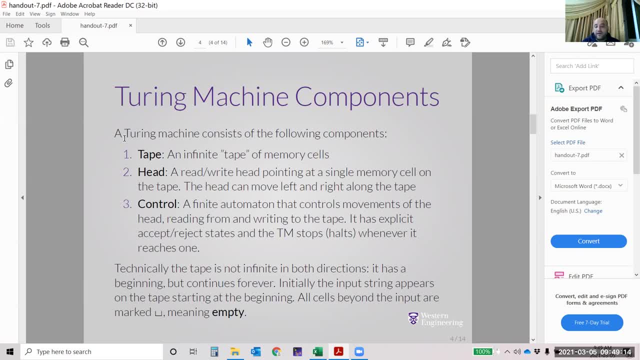 direction. it has a beginning but continues forever. initially, the input string appears on the tape, starting at the beginning. also, beyond, the input are marked like with this simple meaning: if you see this symbol, this is meaning empty. so I have a quick question regarding the tape. so essentially, let's say we are at the middle, but we have. so let me rephrase it. so we have 20. 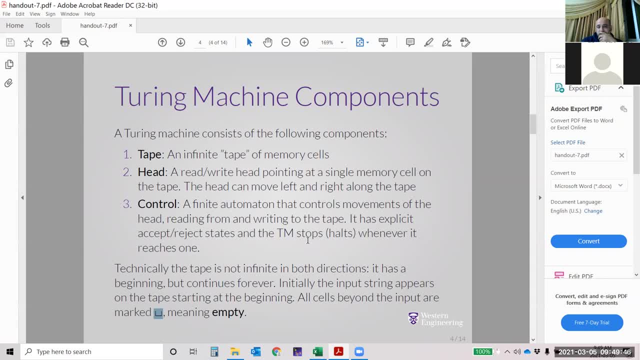 memory cells and we want access 10. would we have to go one by one? yes, it's a table, okay. so essentially speaking it's like stack, but without getting rid of the part at the top. So we can just-. Yes, you can go left and right. 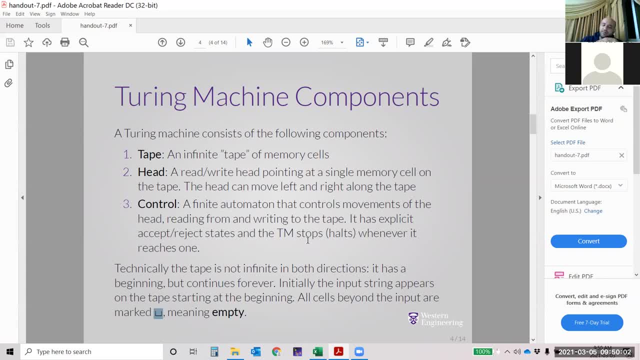 Okay, But you have to move one memory cell at a time. Okay, it's not like. okay, gotcha, I need you to imagine. do you know the normal tape that we used here in nineties? Yes, the-. So if there is a song at the middle, 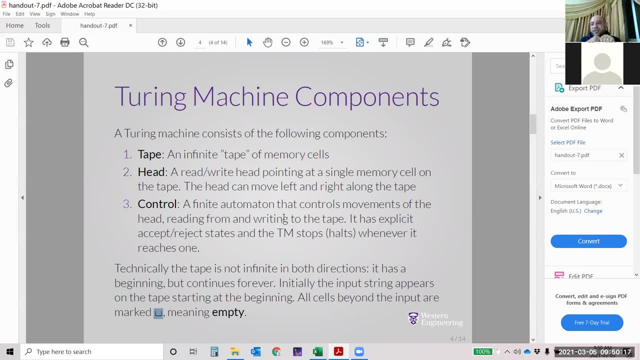 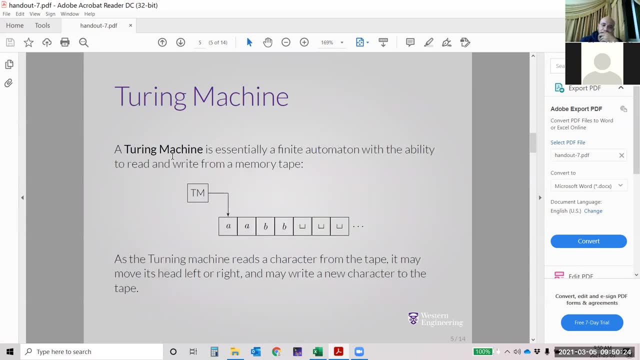 you have to make forward all the way till you reach it. Okay, It's the same. In order to call the function, would we have to, I guess? so my question is: is it possible for us to specifically find a value without actually using the tape? 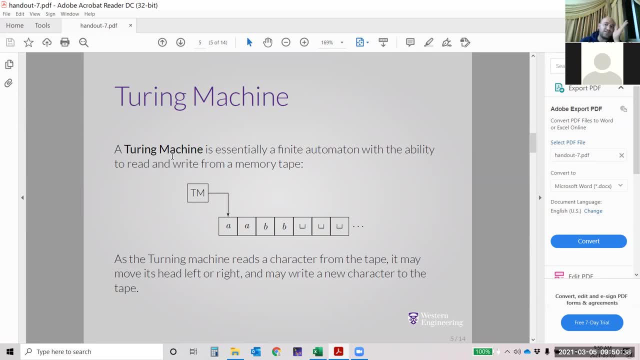 Like: is there a possibility That will be a direct memory access, which is different concept? Okay, Yeah, Okay, A Turing machine is essentially a finite automaton with the ability to read and write from a memory tape. This is the extra thing that give the computational model. 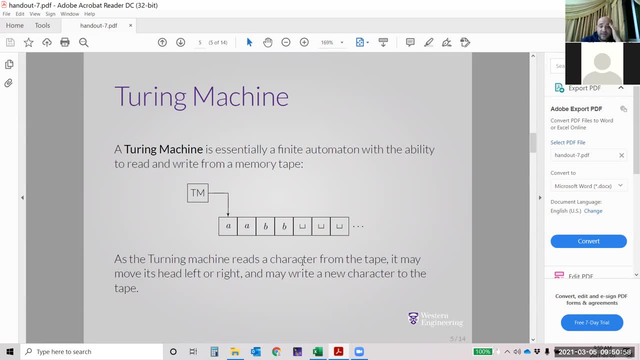 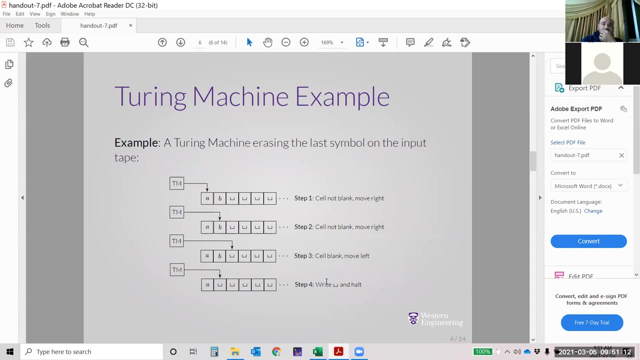 more power. As the Turing machine reads character from the tape, it may move its head left or right and may write a new character to the tape. So it has these left, right, read or write options. Turing machine example: a Turing machine erasing the last symbol on the input. 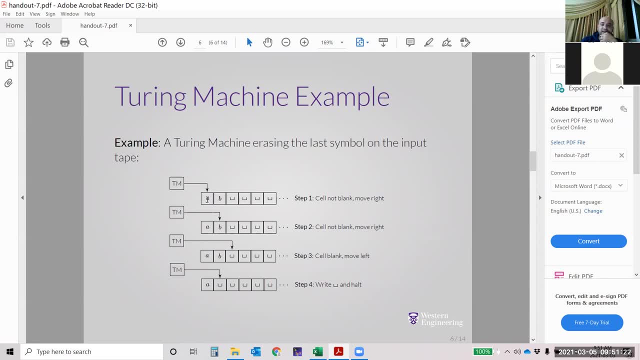 If I have, this is the Turing machine. the tape is at A step one, not a blank move right, Okay, B, not a blank move right. Then I see here a blank move left back. Once I move left, I remove the last bit. 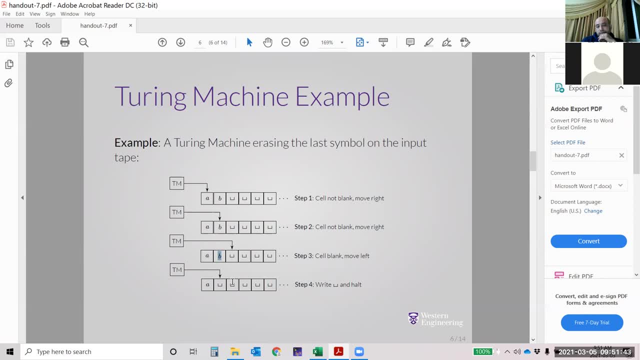 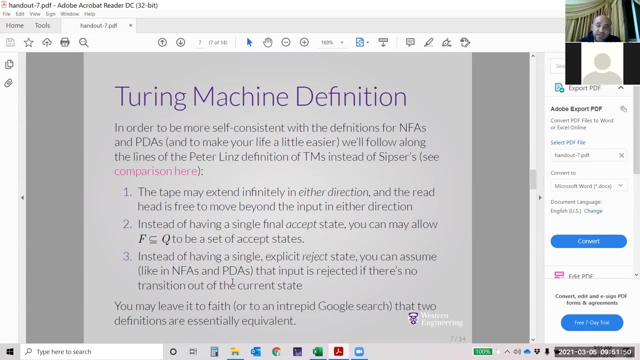 Here how it's working. Turing machine definition. In order to be more self-consistent with the definition of NFAs and PDAs and to make your life a little bit easier, we'll follow along the lines of the Peter Lenz definition of Turing machine instead of Spicer. 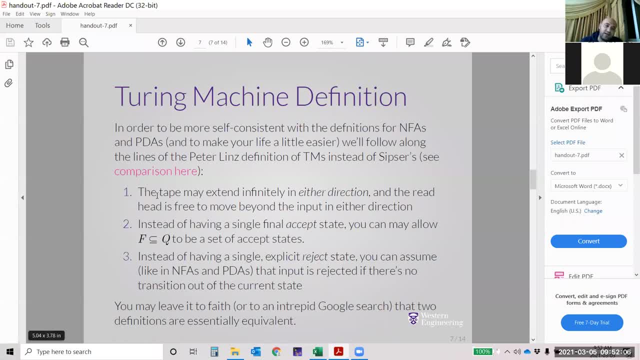 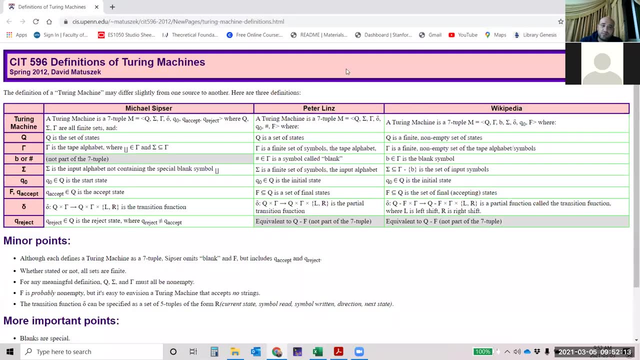 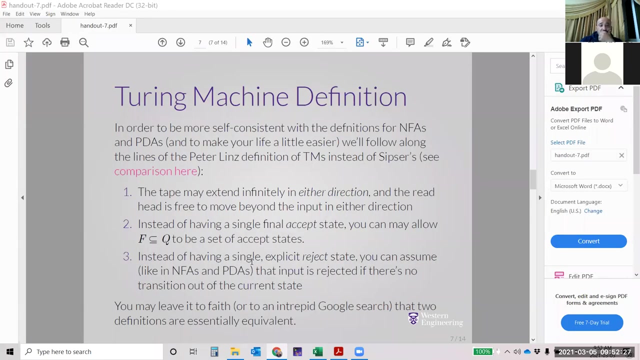 See comparison here. If you press here, you will see the difference, the difference of definition of Turing machine between Spicer and Peter Lenz. Peter Lenz is a bit, a little bit easier. Okay, Tabe may extend infinitely in either direction. 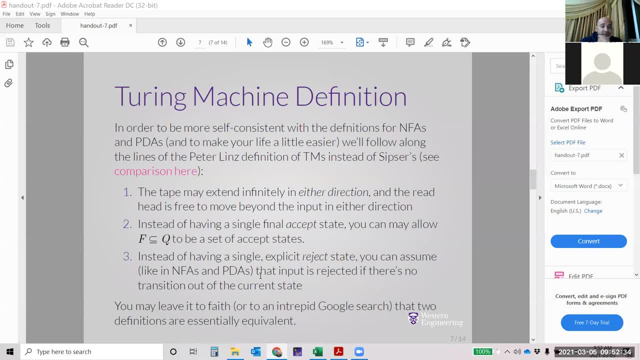 And the read head is free to move beyond the input in either direction. Instead of having a single final accept state, you can may allow F belong or equal belong to Q to be the set of accept states. So Peter Lenz, allow us, in his model, to have more, more, more F. 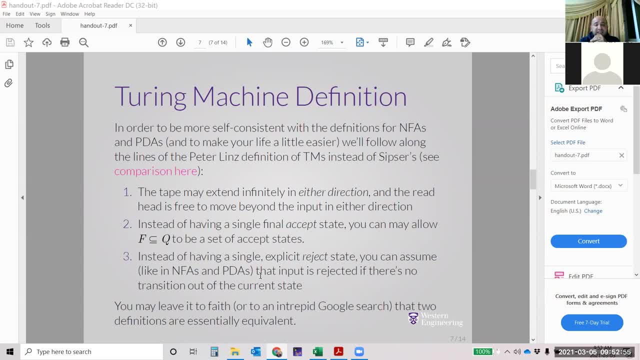 So Peter Lenz allow us, in his model, to have more, more, more F, more than one accepted state. Instead of having a single explicit rejected state, you can assume, like in NFA and PDAs, that input is rejected if there is no transition out. 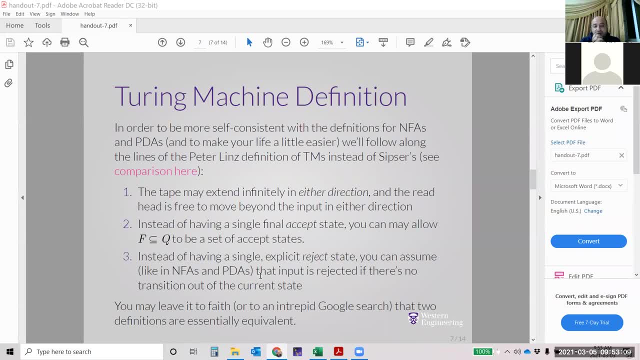 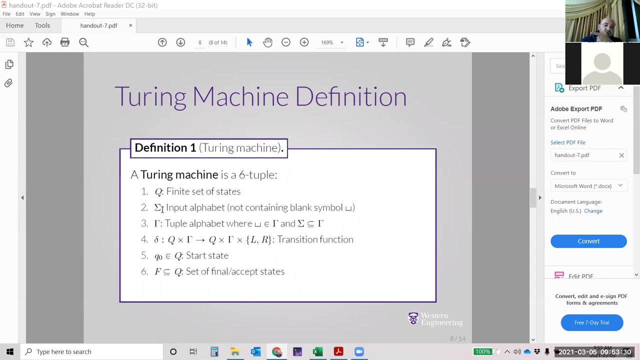 of the current state. You may leave it to faith or to interpret Google search that two definitions are essentially equivalent. They are equivalent. However, the Lenz definition is easier for you to understand. So the Turing machine is a 6-tuple Q sigma gamma. 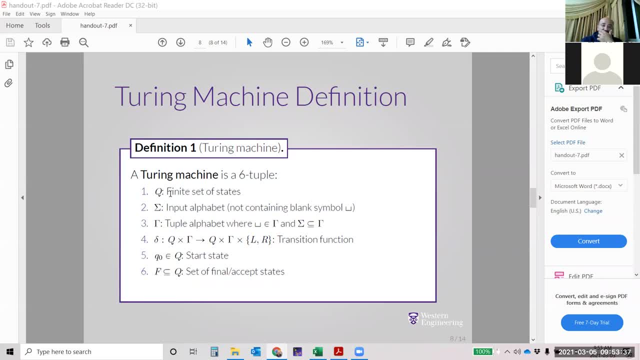 delta, Q0, and F. Here are a finite set of states. This is the alphabet not containing a black symbol. The black symbol is a symbol used to show that this memory cell and the tape is empty, So it's not part of the length of the alphabet. 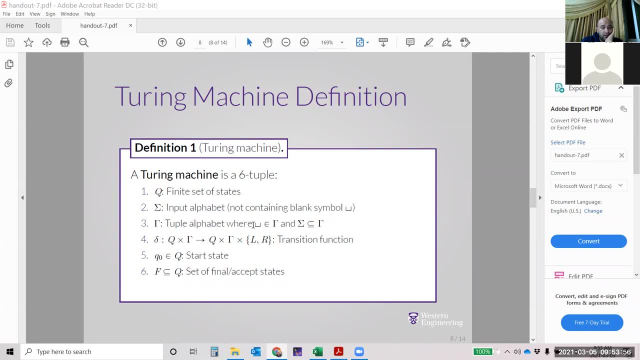 The tuple alphabet, where the black is belong to T and also the alphabet the normal alphabet is belong also to gamma. Delta Q times. gamma will send me to a new Q or to new state with gamma and with where to move left or right. 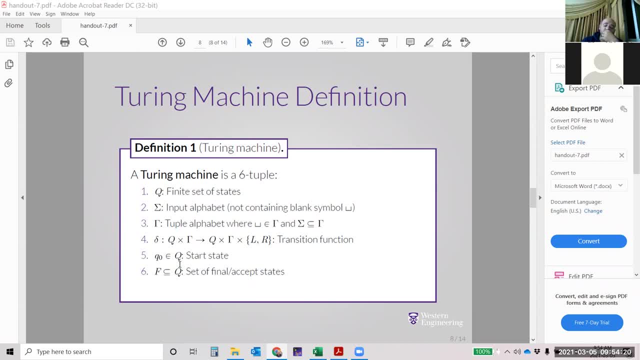 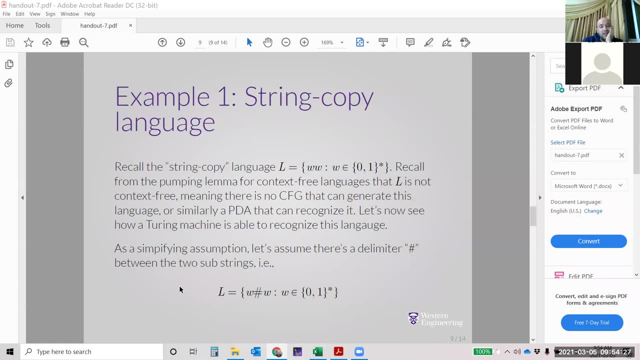 I have to know Q and O belong to Q, which is the start state, and F is the accept state. String copy. Recall the string copy that we took it in handout 6.. And we said that the pushdown automata cannot deal. 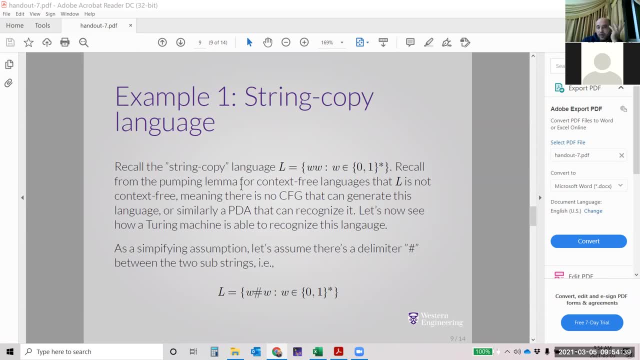 with this kind of examples. Recall the pumping lemma that L is not a context-free. We proved that L is not a context-free for WW just now, meaning there is no CFG. So that's something that can generate this language, or similarly, a PDA that can recognize it. 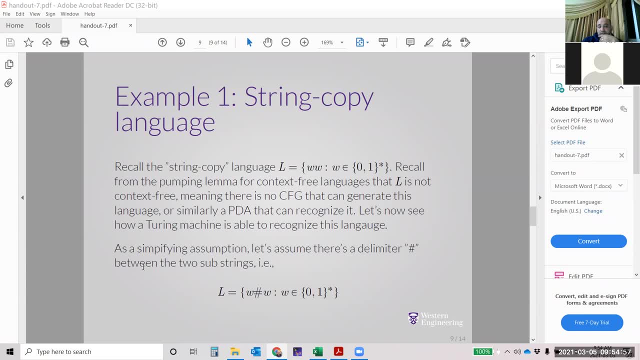 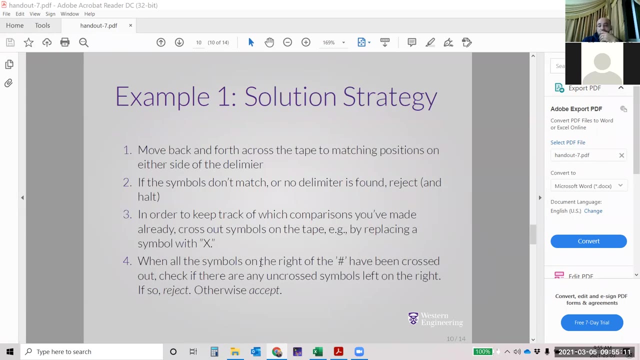 Let's now see how a Turing machine is able to recognize this language. As a simplifying assumption, let's assume there is a delimiter hash between the two substrings. Move back and forth across the tape to matching position on either side of the delimiter. 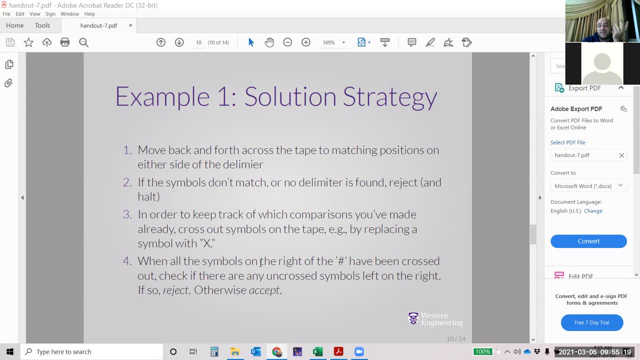 Delimiter. If the symbol does not match, the delimiter will not match. It will not match or no delimiter is found. reject or halt. we call it in uh, in turing machine in order to keep track which comparison you are made. already cross out the symbol on the tape, example, by replacing a: 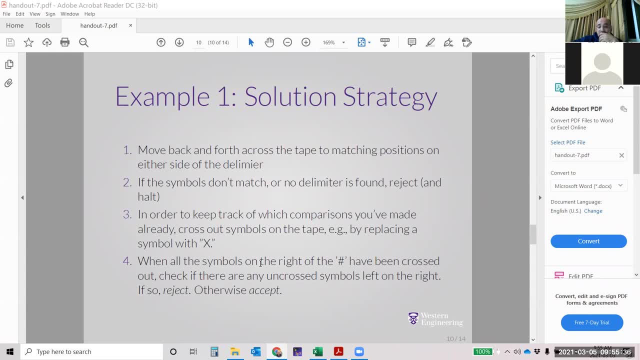 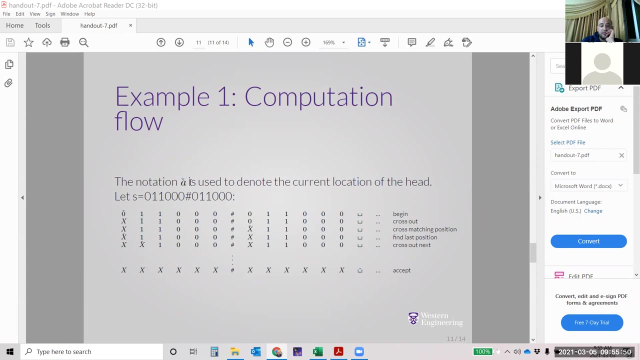 symbol with x when all symbol on the right of the hash have been crossed out. check if there are any, any cross symbol left on the right? if so, reject, otherwise, accept here. so then, mutation a is used to denote the current location of the head. so here we have this one. 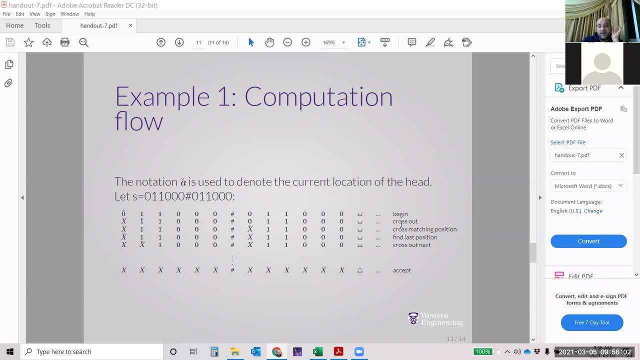 and we will start, and this is the heart, the hash begin. cross out the first one across matching position. fine, you will keep crossing till you reach to this point. if there is no unacrossed cells, then accept. okay, state of transition. let's draw the state of transition diagram for l. 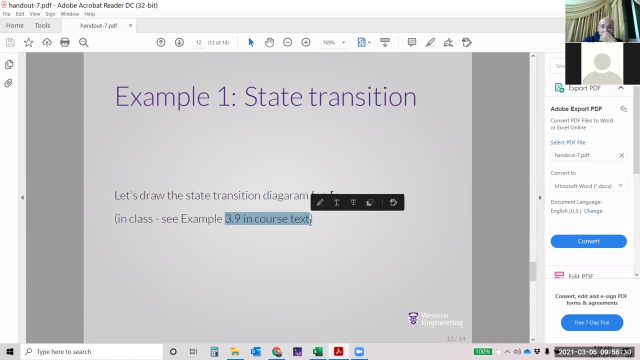 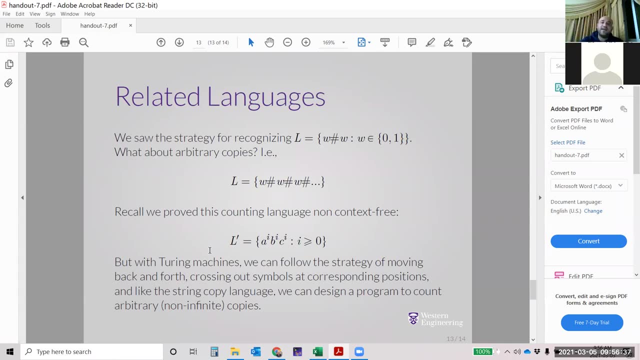 see example 3.9 in your textbook. this will draw the state of transition and next class we will have the class note with more example. also, the ta will give you more example on this. related languages: we saw strategy for recognizing l. what about arbitrary copies if we have multiple w's? recall we approved that is this example a to: 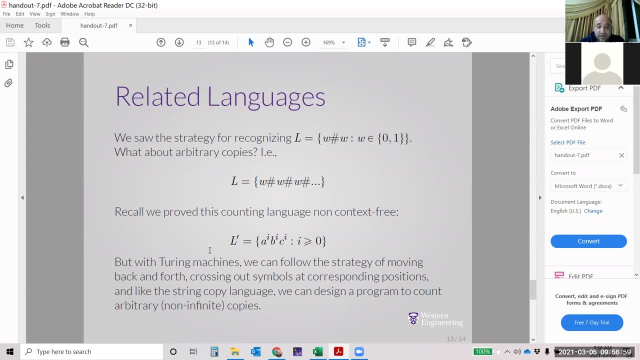 the power i, b to the power i, c to the power i is not a context of three, but with turing machine we can follow the strategy of moving back and forth, crossing out symbol and corresponding position and, like the string copy example, we can design a program to count arbitrary non-infinite. 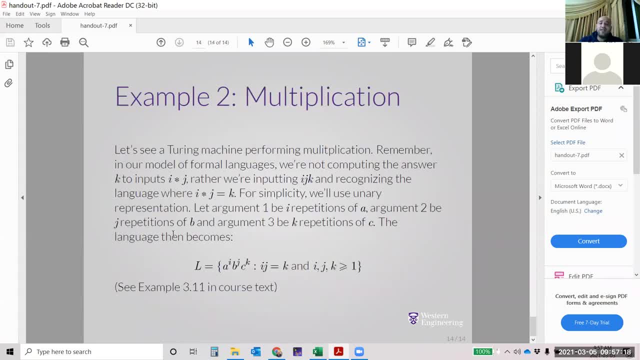 copies the multiplication. let's see a turing machine performing multiplication. remember, in our model of formal languages we are not computing the answer k to input i times j, rather than we inputting i, j, k and recognize the language where i times j, equal k, for simplicity, for. 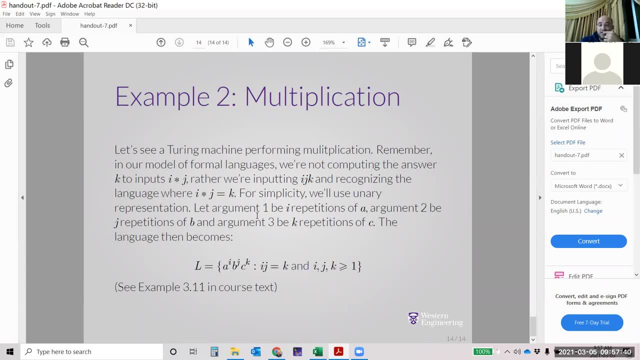 simplicity, we will use unary representation. let argument 1bi repetition of a. argument 2 will be j, repetition of b, and argument eight, as 3.5 will be k, repetition of c. the language will become a to the power i, b to the power j. 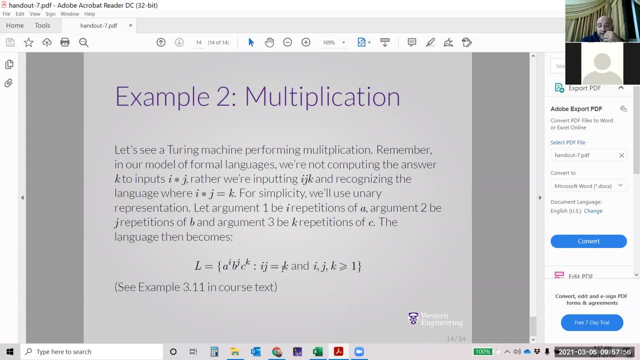 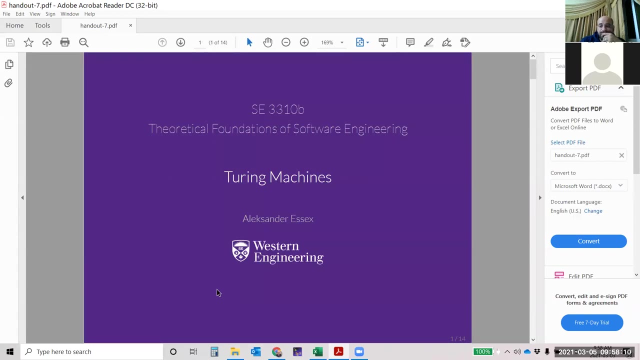 and c to the power k, where i j equal k and i j k greater than one. also for this one, see the example number 3.11 in your course text. okay, guys, questions, questions you have to read. next friday we have a quiz and presentation will. 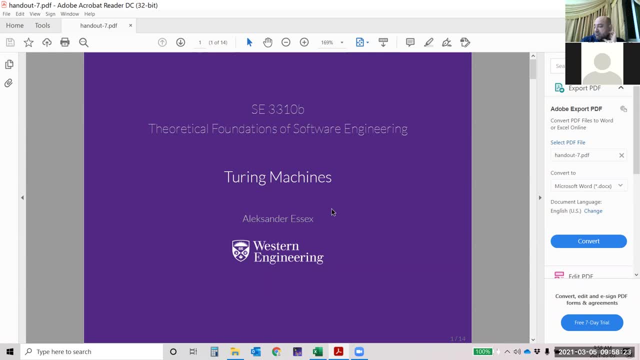 start on thursday we will have the turing machines. uh, class notes. it will not be that much: three, four, five, five pages. there are only five pages: the class notes. we'll finish them in 10, 15. minutes. then we are ready to move to handout eight, which is here. we finish our computing. 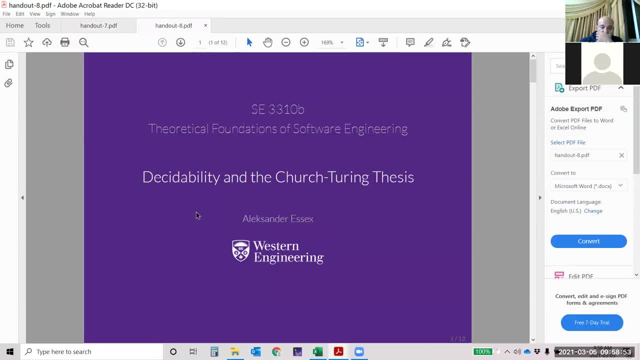 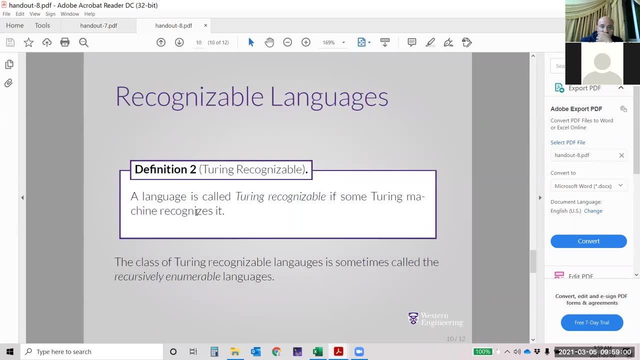 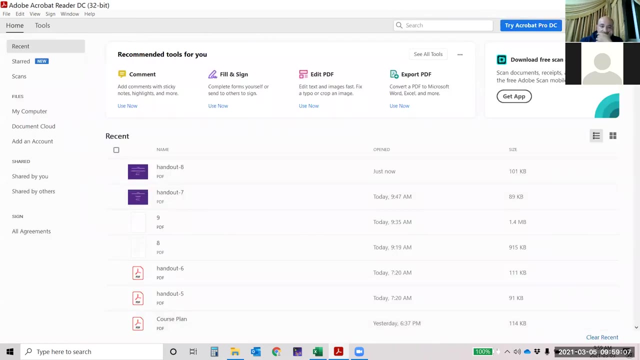 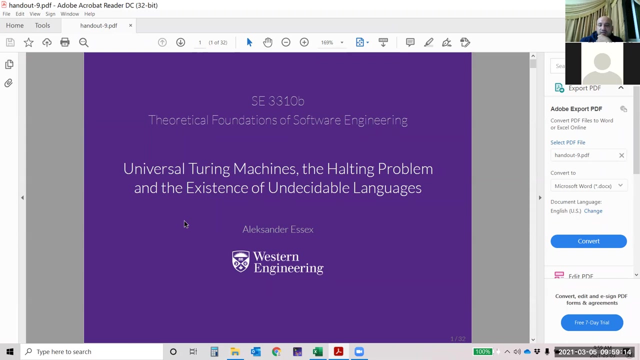 then we'll move to hand out which is decidability and the chair storing pieces. we'll start talk about some the language hierarchy again. then we'll talk some issues in simple way. we'll not go deep details. we'll not go deep details, then hand out nine. we'll go universal: turing machine halting problem and the existence of undecidable.